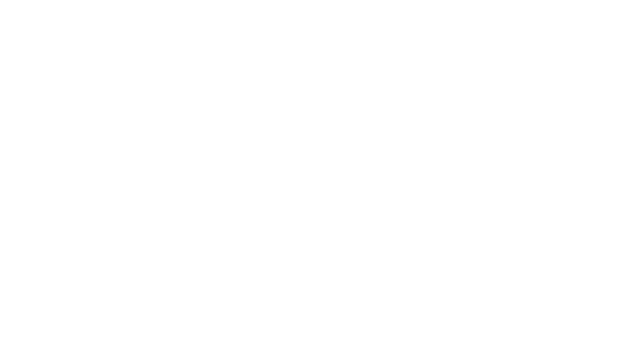 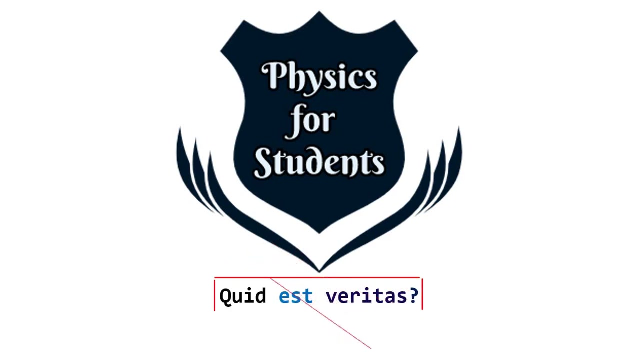 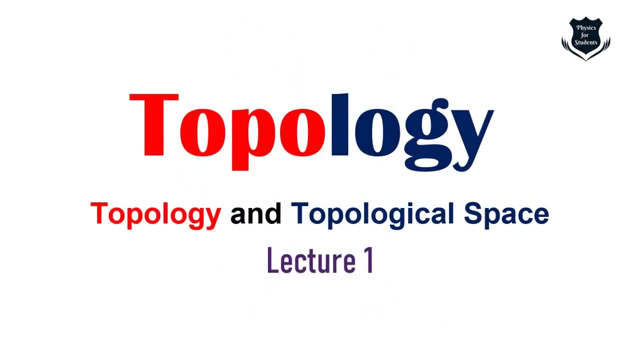 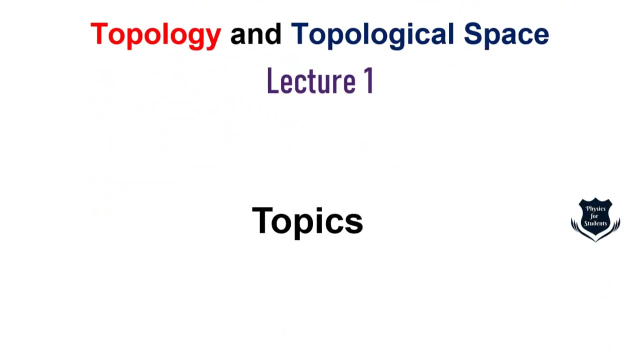 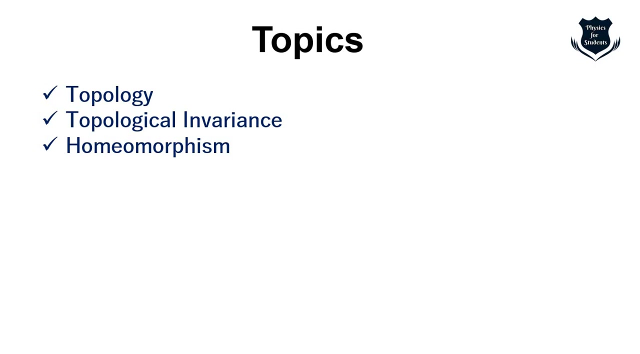 This video is presented to you by physics for students. In this video we are going to look forward on the topics of topology. So the topics concerned are: what is a topology? what is a topological invariance? what is called homeomorphism? what is Euclidean space? what is a topological? 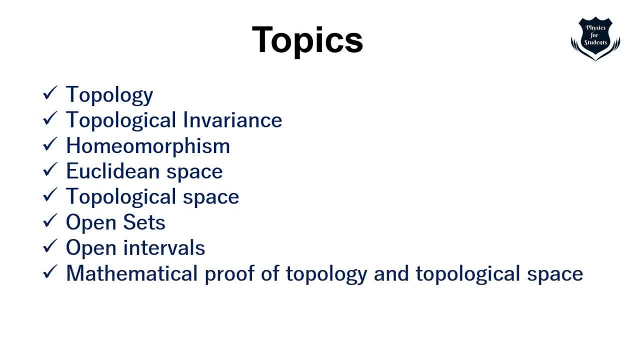 space, what are open sets, what are open intervals and a mathematical proof of topology and topological space. Well, I would just like to tell the viewers is that these are the basic building blocks of what consists of the huge topic which is called topology. This is the first video, so we 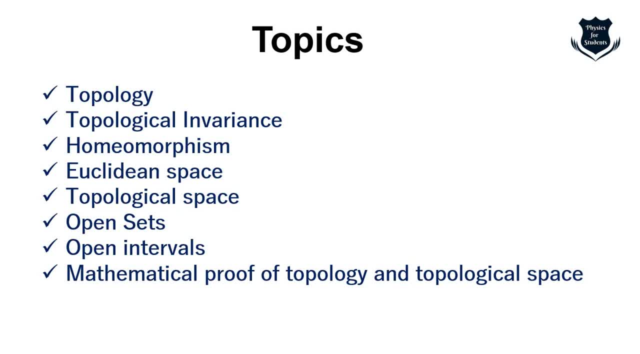 would be looking forward with the basics of topology, and I will try to make it as simple as possible so that, with a basic understanding of set theory and mathematics, people are able to understand the definition and what is called topology. I would also like to tell you that this: 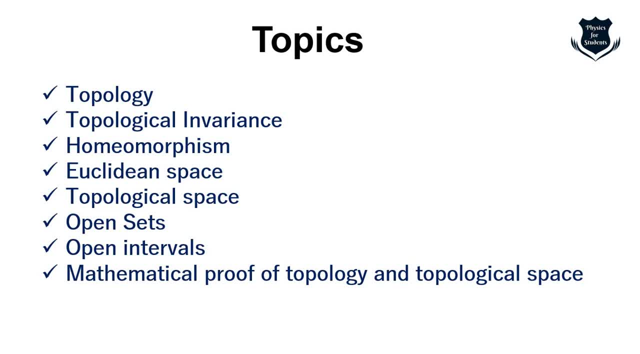 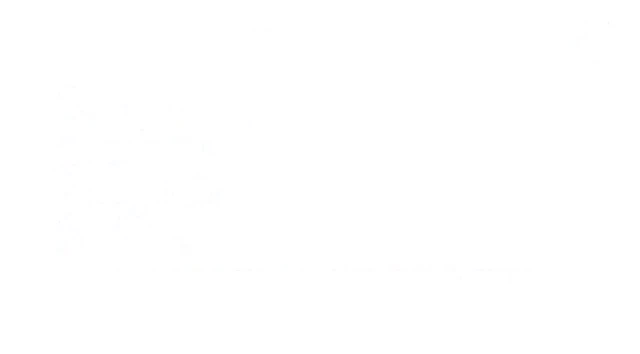 is a very basic idea and a very basic video on topology. The further videos would be dealing with more mathematical intricacies. So to start with, we need to know what is topology. So topology is actually is what we call is the study of shapes which can be stretched, which can be. 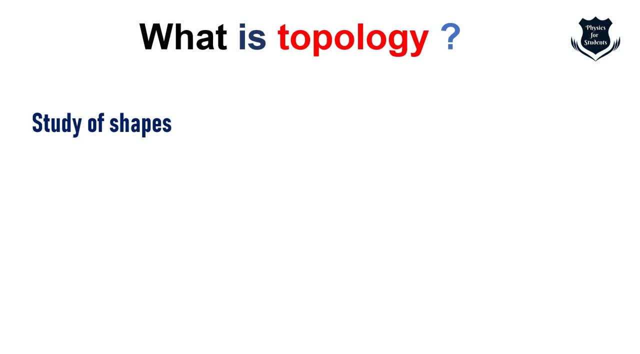 squished and otherwise deformed, keeping near points together. So, as you see right here in front of your screen that these are different shapes. The first one is a cup, the second one is a torus and on the extreme right hand side you can see a small animation where the cup is being. 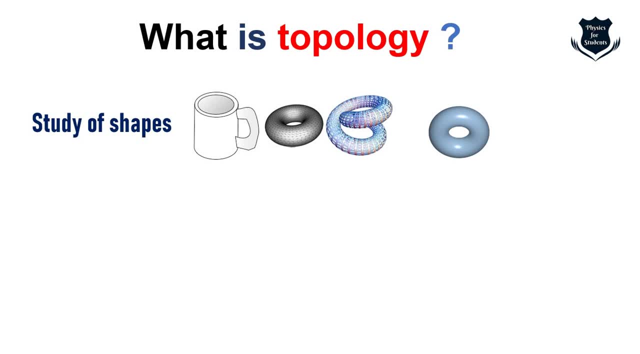 morphed into a torus and the torus is morphed into a cup. Now, this is for those who know topology, who has been studying This is a very common kind of homeomorphism which is viewed in a very common manner. So what we are trying to tell, 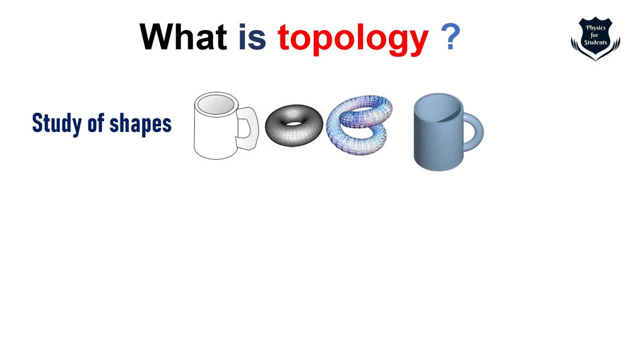 is that it is a study of shapes, and it is. it can be stretched, it can be squished, but keeping near points together. now, nearby or near points is a very undefined term, which roughly means a small neighborhood in a metric space. in a metric space, if two points are located, they are called small. 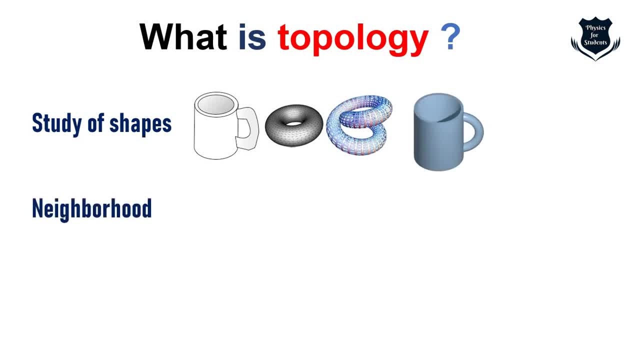 and here we call it neighborhood right. so in this picture you can see a set V in the plane is a neighborhood of a point P. if a small disc around P is contained in V, now this I would say the small disc which is around the V, which is the plane. this has got a lot of implications which we 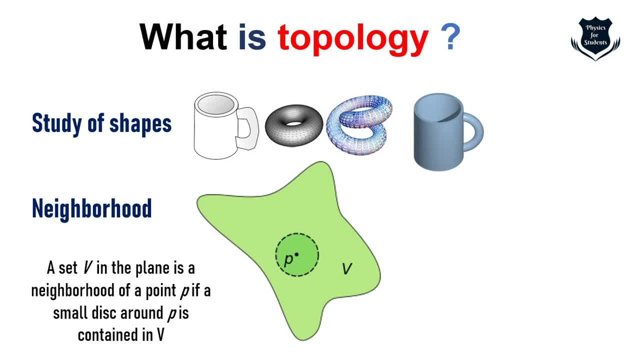 can take it later, which is called a small ball, open ball. lot of things are there, so let us first understood that nearby is an undefined term. right, it is called a small neighborhood in a metric space. two points are located, they are called small and here we call. 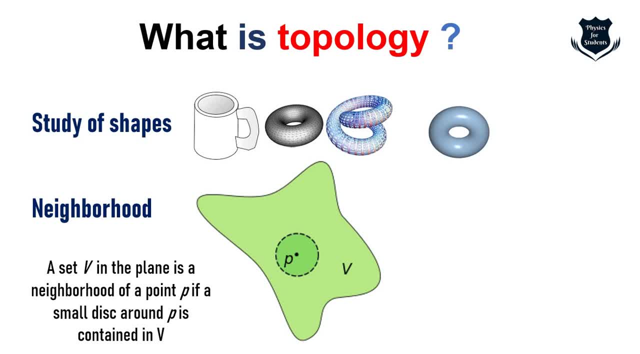 it a neighborhood. so in this picture you can see what I tried to show you. now suppose X is a topological space and P is a point in X. a neighborhood of P is a subset V of X, which includes an open set containing in P. now all these terms, what I am saying right now. my might sound a little bit odd, but these things 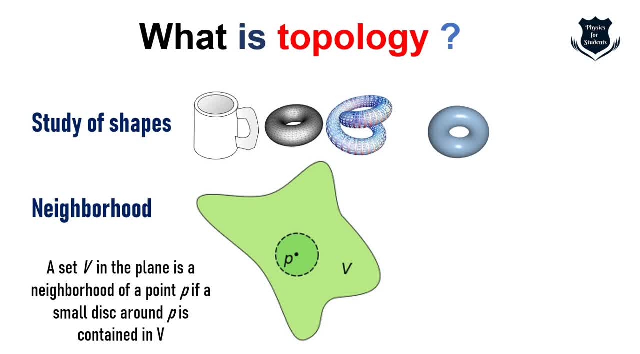 will come clear in the video. so what I told you, mathematically is this right. so don't worry about those terms. it will become clear as we proceed. and now you can also think of this one, as you can move one point around the surface and it should not leave that set right. these things I will be showing. 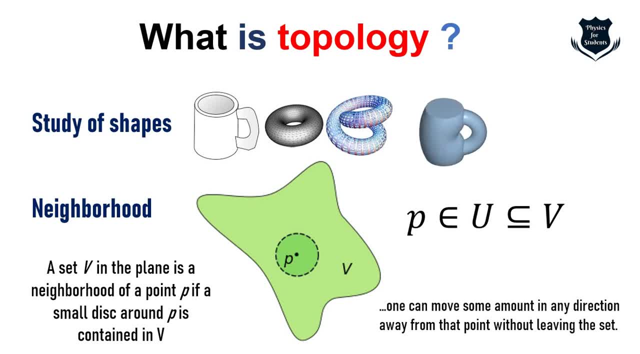 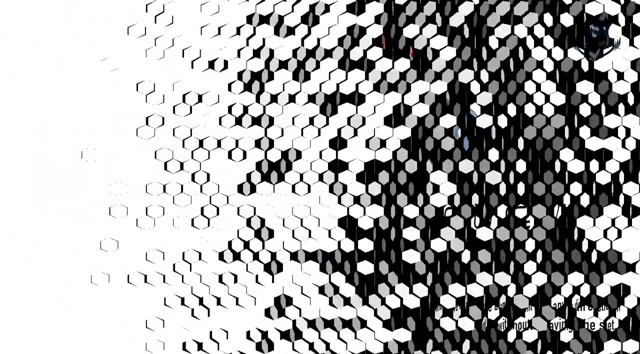 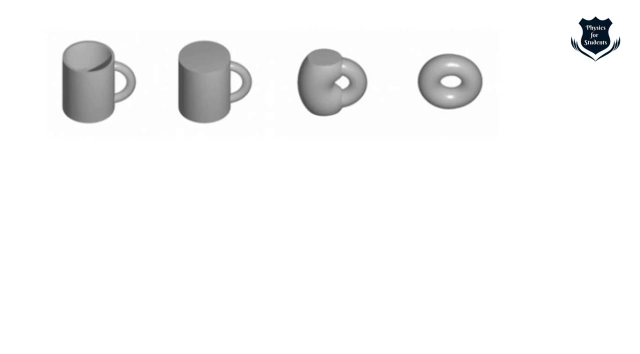 you in a moment. so this is just a basic definition to start with, with a topology and you can think that, if you can, there's a small perturbation and you move a point around a set. it should not leave the set. well, in this particular figure, you see, the property is preserved under homeomorphism. 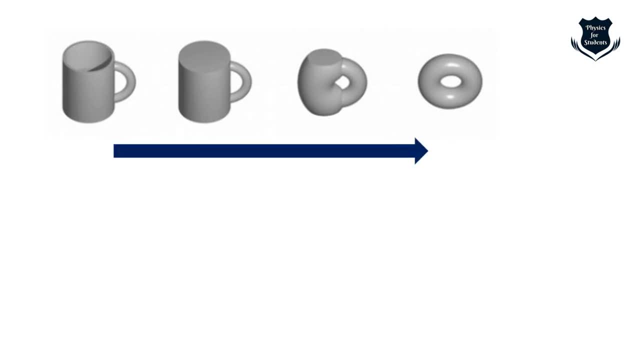 now, what I am trying to show you is that, once this is the form of the outer sleeve and we can see that it did not enter the set, which is just a very small perturbation- and now you can see that it did not enter the set and that was the problem. 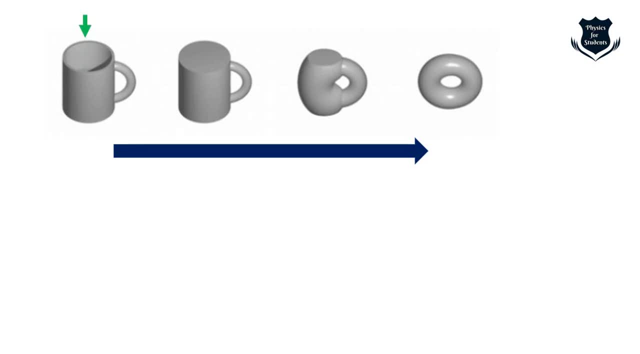 because the whole thing has been modified. it's not going to be the same for any other set, other sets, and it is well preserved so it is. it is also very difficult to find a similar shape, and then the problem is with this is also quite, quite Machine learning in this particular case. 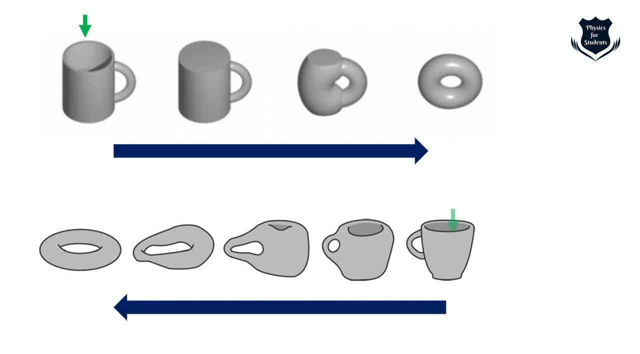 you need to understand that I am not saying that this is because this is not a very good shape. so why am I not saying it is not a very good shape? you can simply think about the shape. the shape will be different and the shape will be a little bit different. 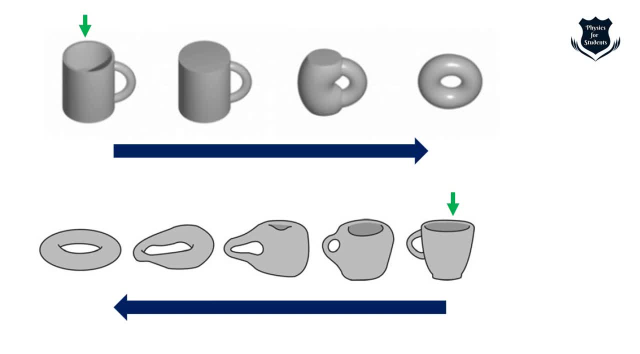 and so this is the design is not based on the shape. trying to tell you is that even if you mathematically consider this to be a function which is a cup and it is being undergoing homeomorphism and is become a torus, the reverse of the function is also true. that means the torus can again regain into a cup. So here you see, the 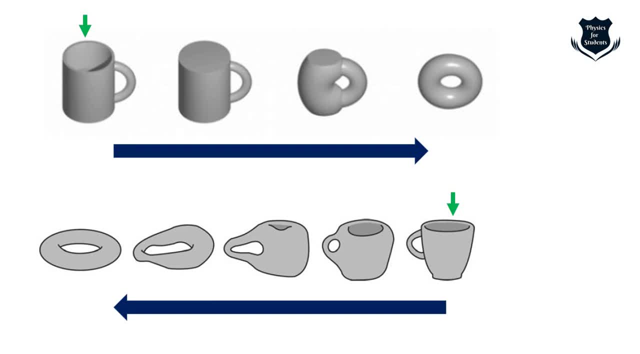 property is preserved under homeomorphism. right now, you can just think homeomorphism as a corresponding between two figures, such that the function and its reverse are continuous. Now I have shown, if you have seen, my first video where I have used certain clay materials in order. 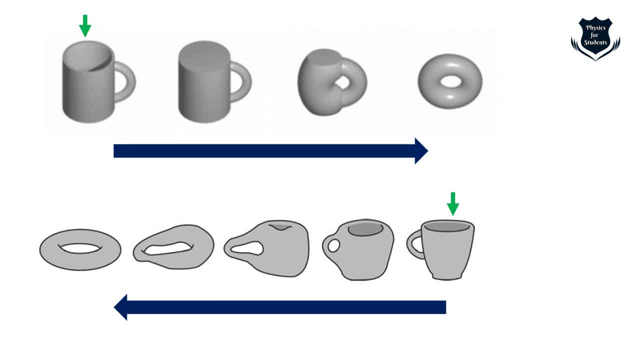 to give you a basic understanding of topology. tearing and gluing is not allowed right, but the thing is that that is entirely not true. There is something which is called a dent twist, which we will come forward. is a topological move or a topological 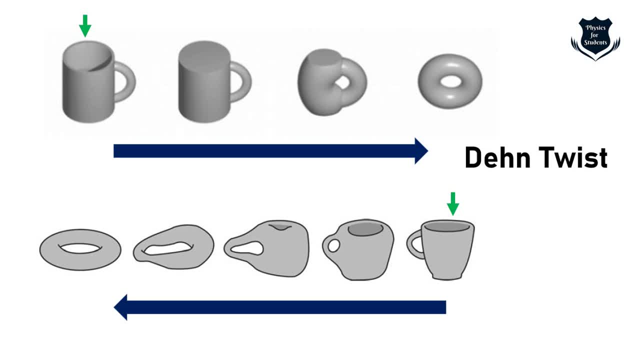 I would say yes, a move that cannot be achieved without cutting and pasting. so I I would like to tell- I have given the First video of mine in the description box, where you can see what I have told- that this can be changed without Gluing or without tearing. but that is not true. 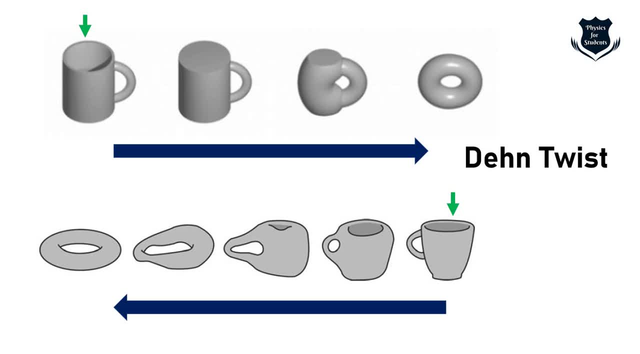 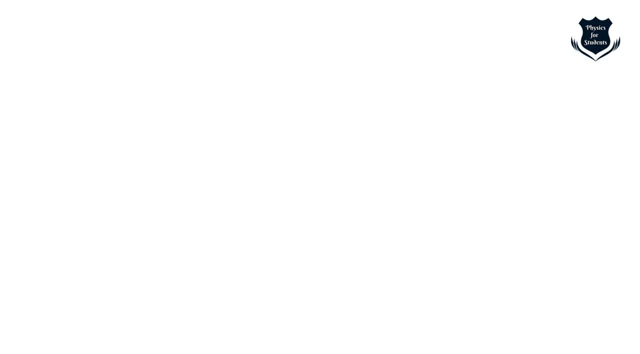 There is something which is called dent twist which makes things like that, and we are going to see forward in this video. Now, If, in this particular Form, if you see a very rudimentary sketches where these triangles we have learnt in school days. This is what we call congruence. See, this is side, side side. 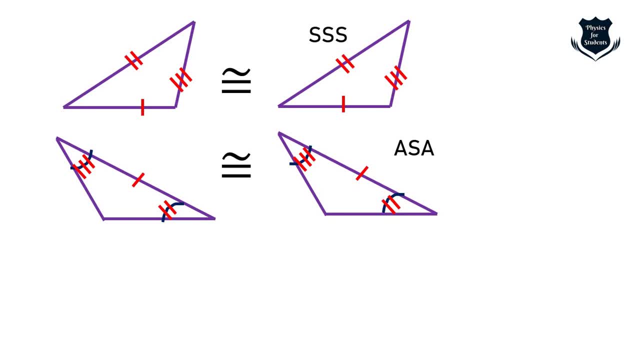 Then we have got this angle side and another angle, then we have got this RHS. All these are basically what we are trying to tell. they are congruent to each other, right? So what I am trying to Tell you is that when we speak of Euclidean geometry- 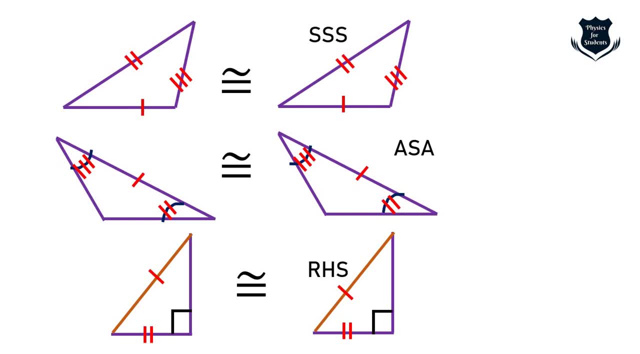 There is a concept of what is called congruence, right? So once we tell the concept of congruence, two shapes are congruent when one can be mapped with the other, Right? so I can take it in this way Why I am explaining Euclidean geometry right now instead of topology. things will become clear. 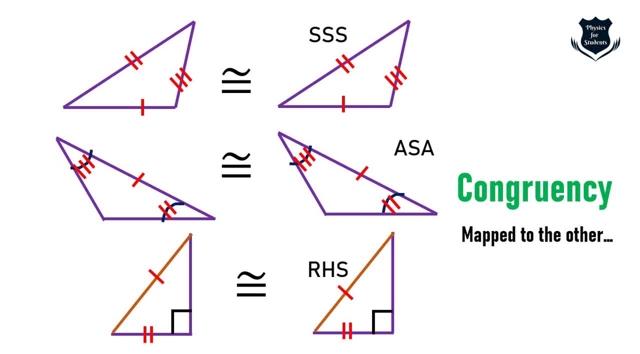 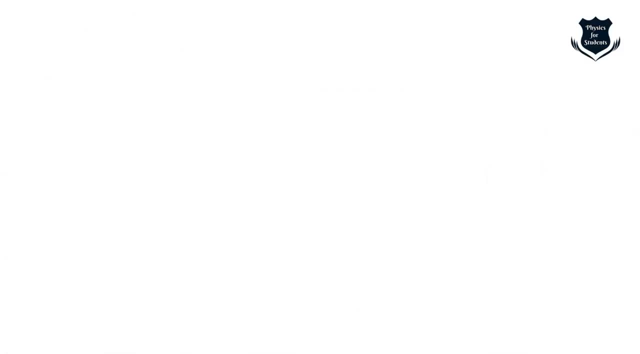 But congruency is something which we call that two shapes are congruent when one can be mapped into another, which you can see. that The simple sketches of triangles, right-hand side, and asosceles shows how they are congruent to each other. If I take this part of the 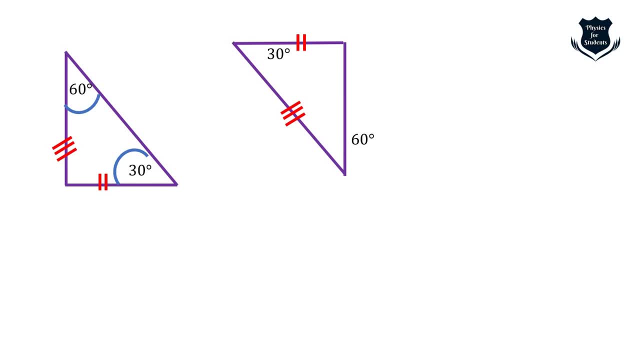 Video where I am trying to show you this. then two ships. as you see, the first left hand side, right angle Triangle has been rotated in this direction and has taken this shape right, and also this angle I have just taken, abrupt 110 degrees, can be taken into this right. so now you see here, angles do not change when you slide. 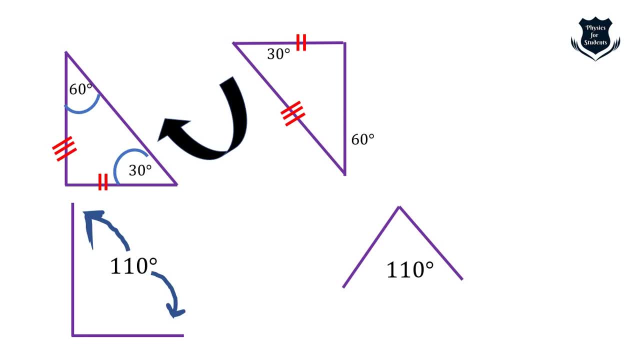 and rotate. however, no deformations or twists are allowed. so the first figure is rotated, the second figure is rotated. yes, and you see, angles are congruent and there are no changes at rotation. so this is a typical kind of a property which we see when we are undergoing euclidean geometry. 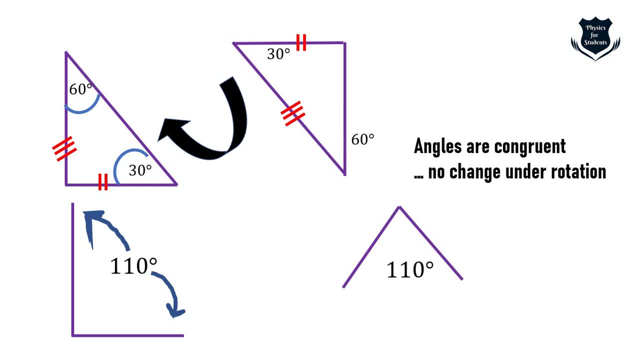 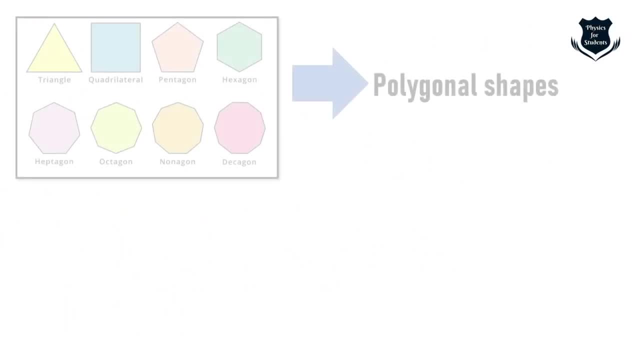 that is under rotation or when we are flipping around, the angles are congruent. the concept of congruency, now, what i'm trying to tell you here is that if you see, in the left hand side, all these can be termed in a group called polygonal shapes: right triangle, quadrilateral, octagon, nonagon. 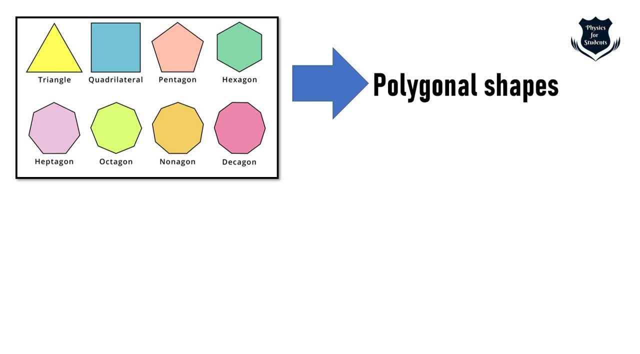 decagon, hexagon, pentagon, heptagon- everything can be grouped in as polygonal shapes. so the first idea which we are learning in topology is that this polygonal shapes can be changed to any other shapes. right, so it can be squeezed, it can be stretched, it can be morphed into any other things. 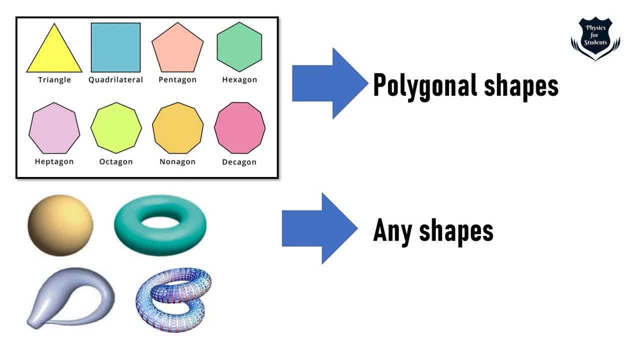 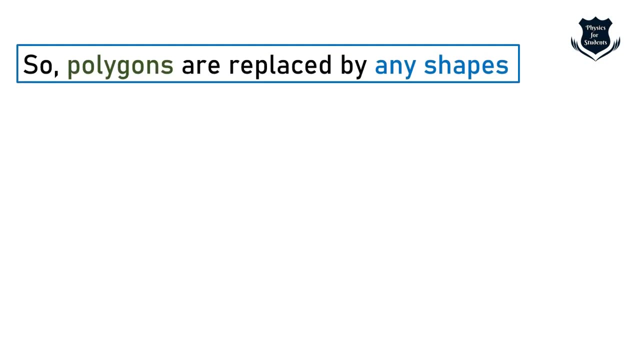 and this is the first difference that we need to know- that from polygonal shapes we are now shifting our idea and knowledge and everything into any kind of a shape, and this is particular to topology. so now you see, here, polygons are being replaced by any shapes, right? so this is the first when we are venturing in the arena of 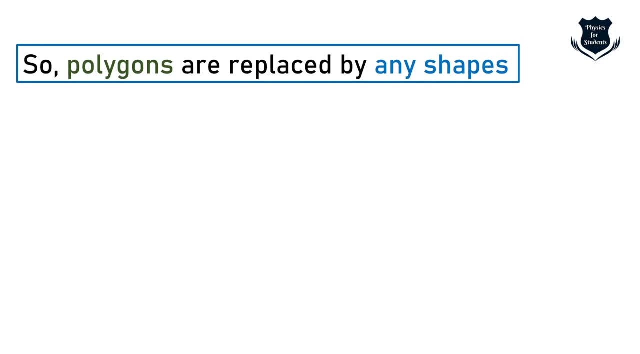 topology. polygons of typical euclidean geometry are replaced by any shapes, and congruency is replaced by topological invariance. now, by topological invariance i'm trying to mean is a property of topology which is invariant, that means it doesn't change under under homeomorphism. so now, 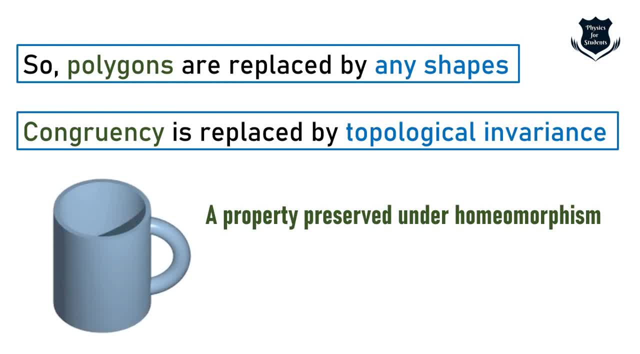 take this right: if you sleep closely. when this cup is now being undergoing homeomorphism is turned into a torus, the property of the near points are being preserved, right. so congruency is replaced by topological invariant. that means i think you can understand in in euclidean ship when we say: 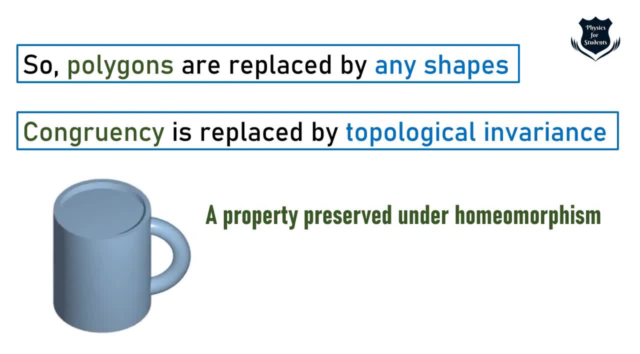 this ship is congruent to this? it is. it is some kind of a similarity that we are doing drawing, but in topology we say that it is topologically invariant. that means it is similar to congruency, but not congruency but topologically invariance, and it undergoes homeomorphism, but the properties. 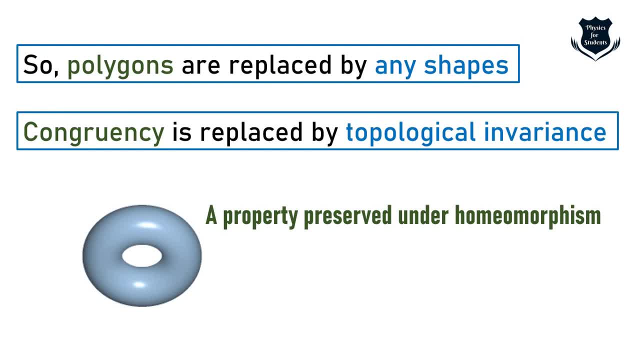 are preserved and the polygons are now being used and now being taken care with any shapes. now i can call uh with a simple example: this torus is congruent, or i would say, topologically invariant, to this cup. so this is the way in which we are going forward with uh: how to pull from euclidean space. we are 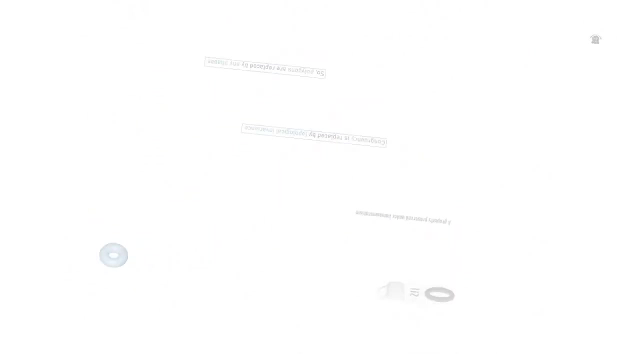 migrating to topology. now, technically it it would be this: if a space x possesses a property, every space homeomorphic to x has that property. what do i mean by this? let me just take you a quick, simple example. so if we have something like this, okay, a rubber sheet. we call topology a rubber sheet geometry. so if you get a 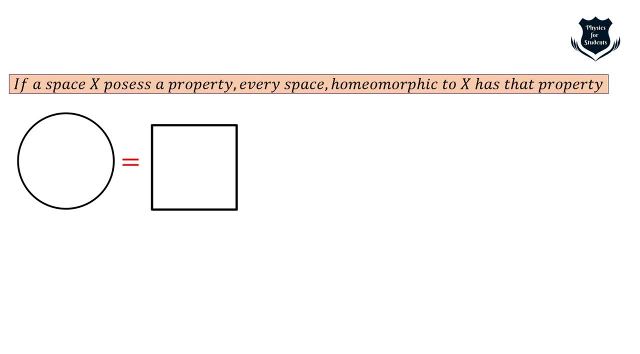 rubber sheet or a clay, in which a circle is equal to a square, which is equal to a rectangle. so we can squish it, we can stretch it and we can do whatever we want and we can turn the circle into a square and then further the circle can be turned into a rectangle. so the property, if you see on the 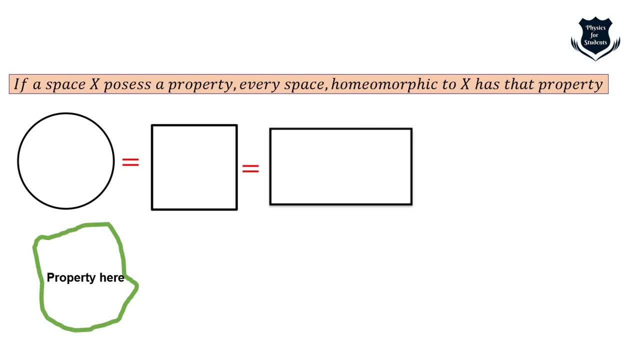 left hand side of your screen. i've just drawn an abrupt figure, so the property on the left hand side, below the object which is in green, will be equal to the property which is something like this, which has been crushed or which has been, uh, undergoing homeomorphism, and which will be also equal to this right. so this is, uh, what we call. 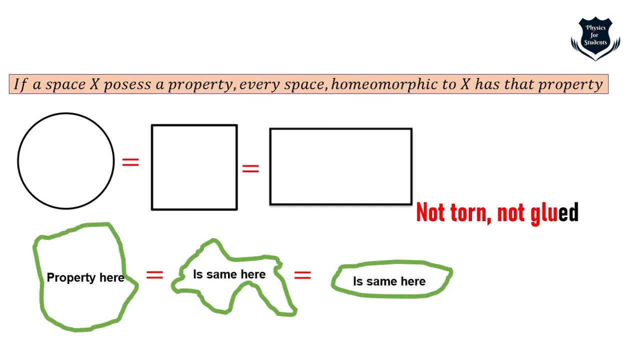 but yes, it should not be torn or it should not be glued. but this is entirely not true for the basic of topology. just to start with, let us assume this as an axiom: it should not be torn or it should not be glued. further topological advancement tells that it can. 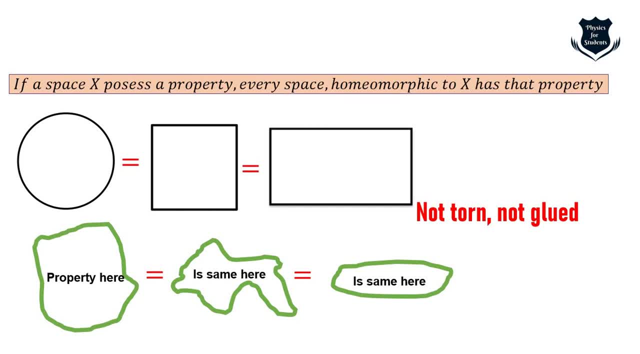 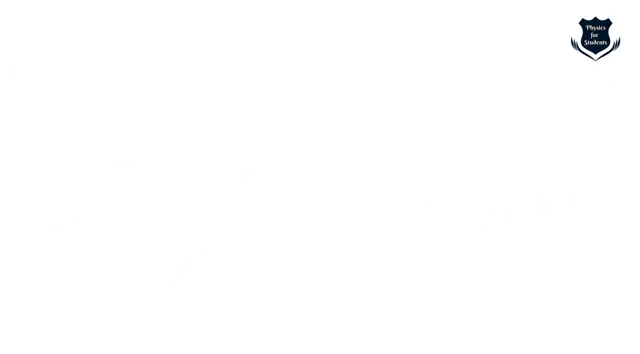 be done. so i think this part is clear once we are done with the first part of the video: how the space possesses a property undergoing homeomorphism, it is preserving, and how the circle is turning into a square and then further into a rectangle- now i can also call this as a torus- and it turns. 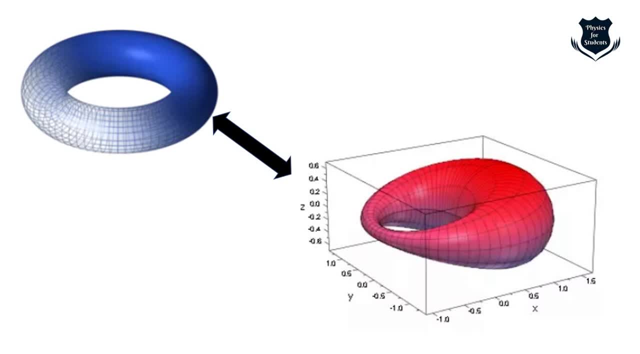 into this right. you see, the topological invariance is maintained, which is formally defined as this bi-directional mapping of one ship to another, which preserves the notion of points being near to each other. by bi-directional, i have shown the arrow on both sides, so it should be on both. 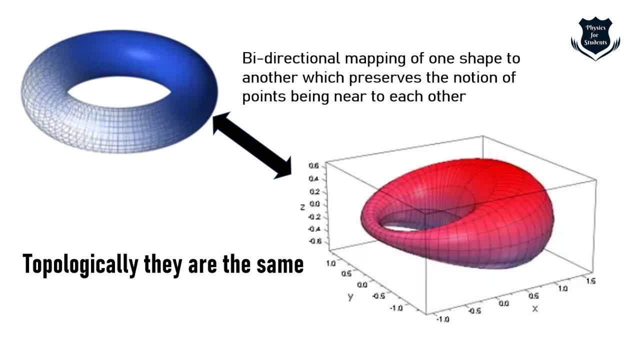 so this torus which is on the left hand side of the screen, marked as blue, is topologically the same as this one, which is a little bit different. so this is, uh, what i'm trying to show you: that they are topologically, they are the same. 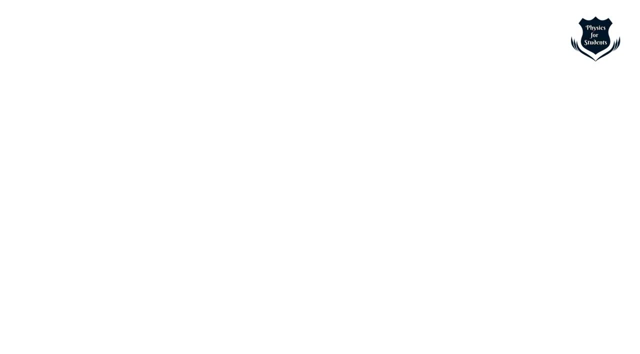 so now, if we have a rubber band or a clay, we can form a circle, ellipse, a square or torus, anything. these very different are very different in terms of geometrically, but topologically they are the same. so these shapes- we told that polygons can be this, this, this, this. 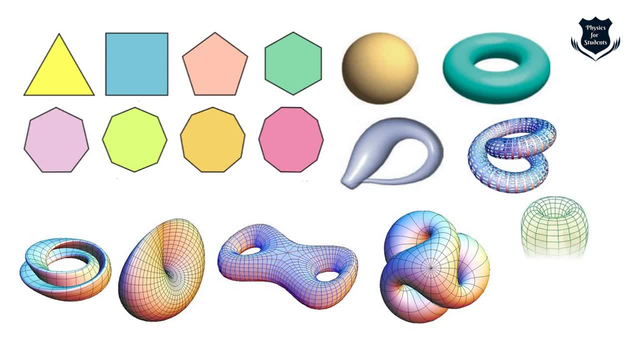 they are topologically the same and those who do topology now can recognize right on the right hand side. this is what we called a klein bottle. so, in case that you have a rubber or a clay about what i have shown in my first video, you can. you can do this kind of morphing in which 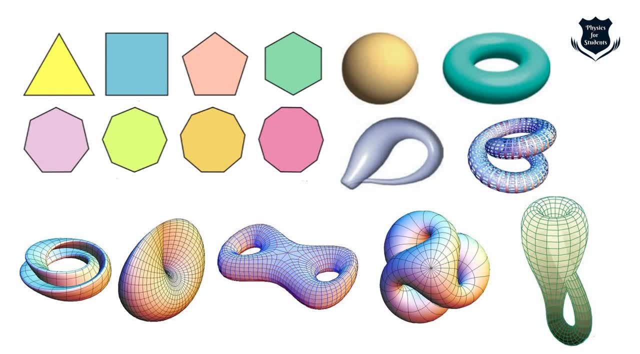 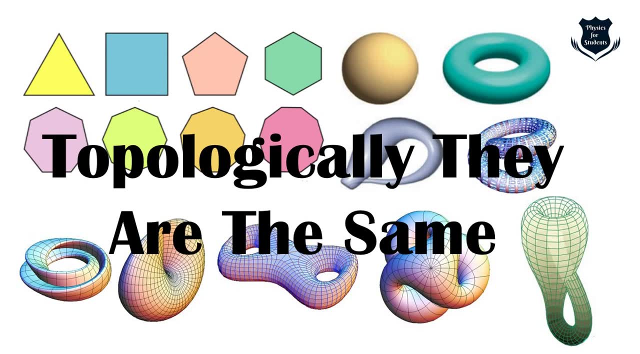 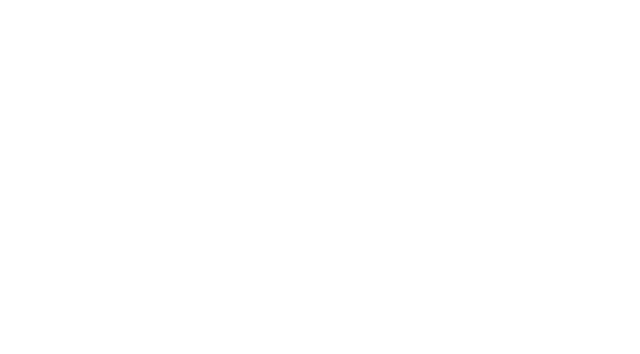 you can start with a triangle and you can come down to a hectagon or anonagon and these things are, topologically they are the same, although geometrically they might be different, but They are the same. So, if I take a little bit more technical, this was a kind of a more of a visual and intuitive approach. 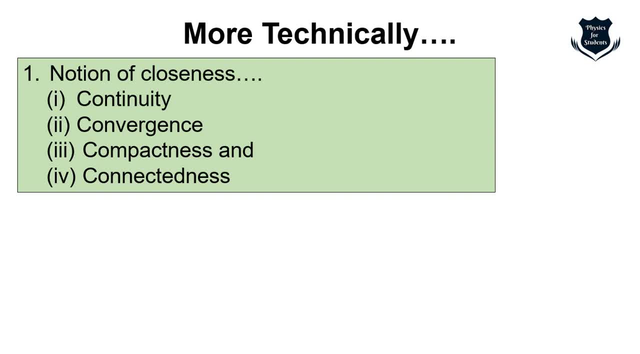 But if I take it more technically, I can call this: the notion of closeness is now is defined by continuity, convergence, compactedness and connectedness. Now this point, number two, I can expand a more what is called convergence and why the concept of calculus continuity is more taken up in topology. 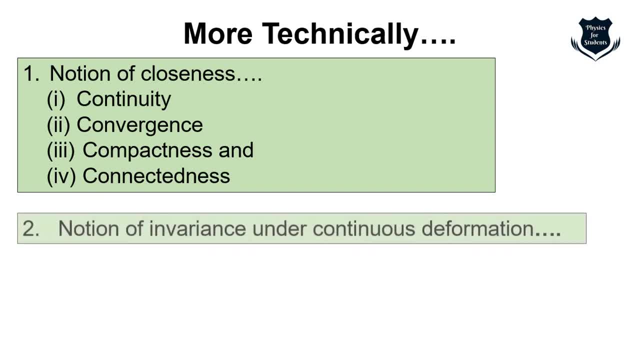 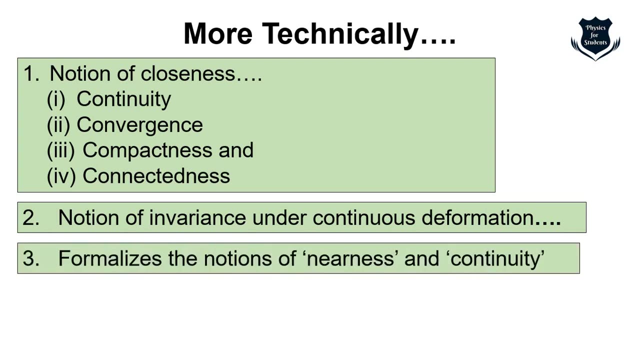 But anyway, this is not the right video to tell you on that. We can call the notion of invariance- That is what we told- that the Euclidean concept of congruence is replaced by invariance under continuous deformation. Also, it formalizes the notions of nearness. 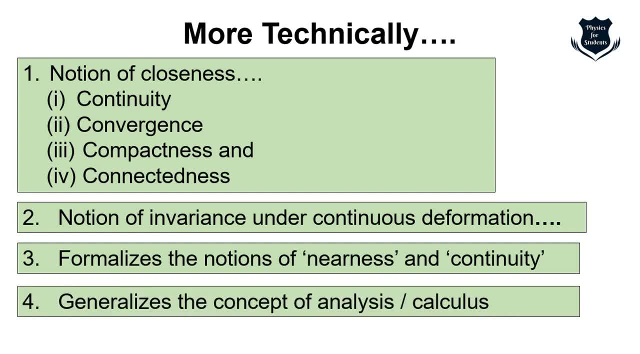 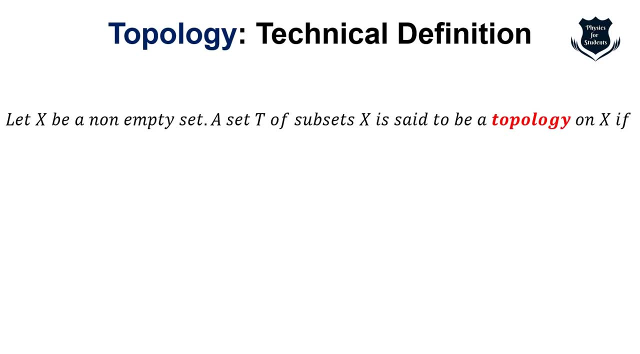 And continuity and it generalizes the concept of analysis and calculus which will be- we can take it up later in some other video. So the topologically we can tell the technical definition as this: If X be a non-empty set, a set of T subsets, X is said to be two. on topology, 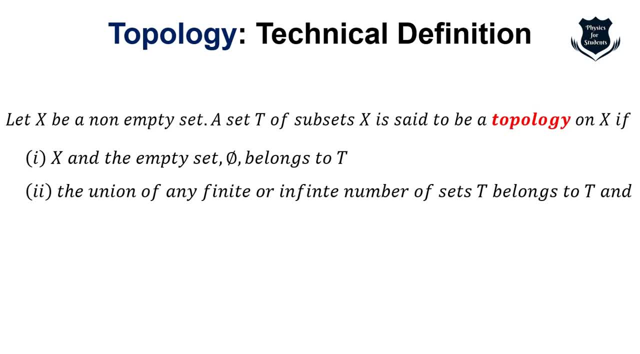 If one X and empty set five belongs to T to the union of any infinite or infinite. If one X and empty set five belongs to T to the union of any finite number of sets, T belongs to T and the intersection of any two sets T belongs to T. 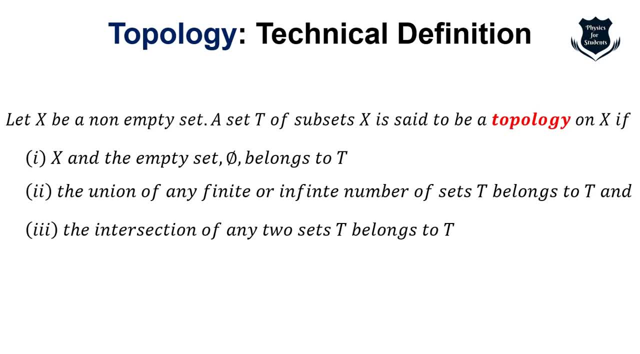 Now, in certain textbooks you might find that T has been replaced by Tau, the Greek number, the Greek letter Tau, but for simplicity I have just kept it T. So this is the three I would say points until they are satisfied. we cannot say the subsets of X to be on topology, on X, right. 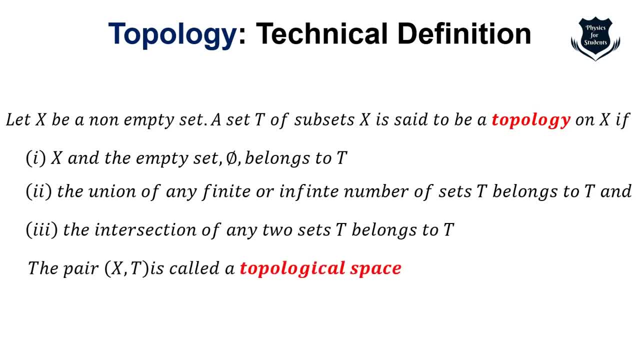 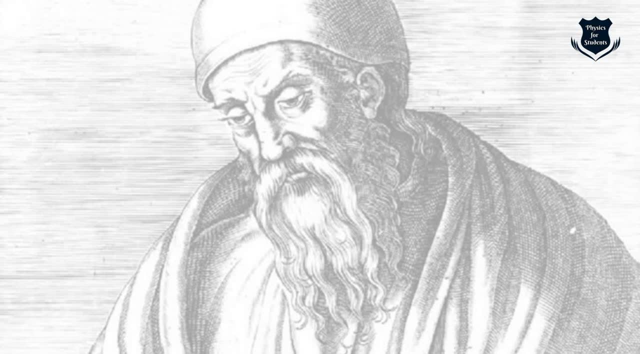 So three thing emerges from this. The pair- yes, the pair- X comma T is called the topological space. one is union, the second one is intersection and third one is water open sets. Now, before I go ahead with this great figure, what I would try to tell you is that if you have been observing my video, then you might have noticed that what we are doing is that we are trying to generalize things. 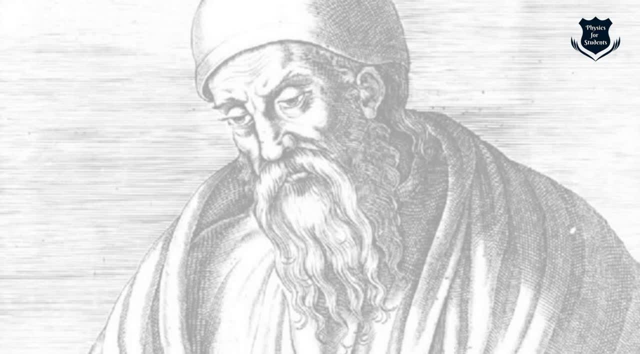 So I mean to say by generalization, if you know that Newtonian mechanics has been generalized more into general theory of relativity. geometry is being more generalized now into topology. the 2D surfaces now are being generalized more into 3D. the surfaces are generalized into manifold called Riemannian manifold and everything. 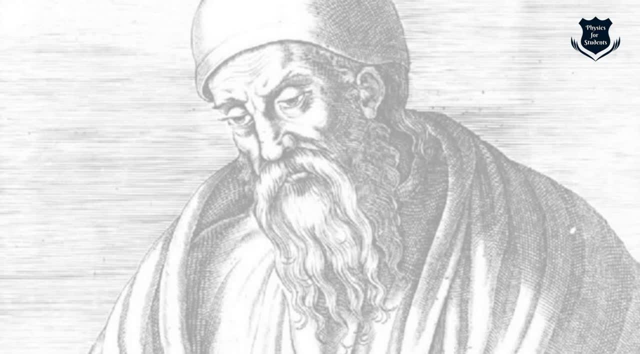 So what I am trying to tell you is that, with the advancement of science and mathematics and the different branches of mathematics, group theory, relative theory is also being generalized, ring theory, knot theory, topology- whatever we are learning, we are going more towards unification. 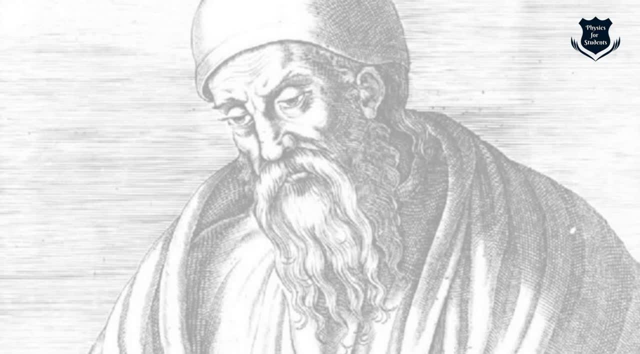 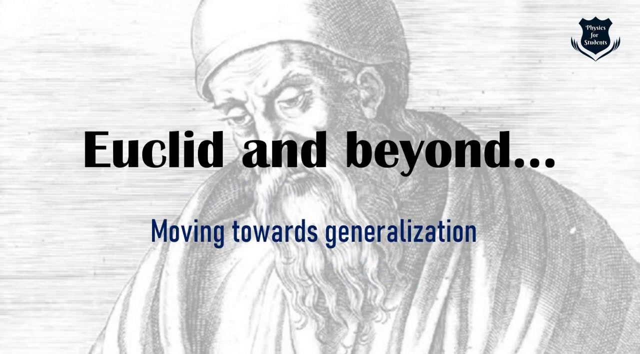 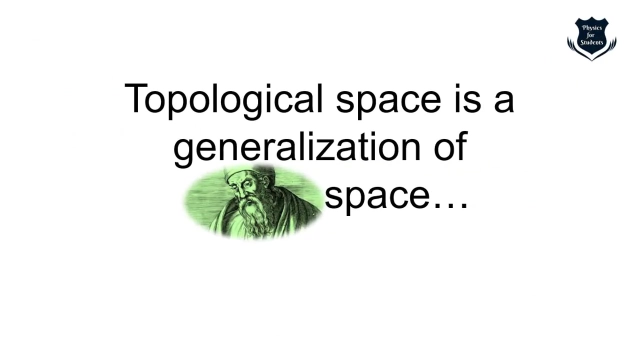 or I would say it is more towards generalization. That means we are trying to generalize things easier so that in one particular theory we can explain everything. Okay, so you might have recognized this very famous figure. It is that of Euclid, So topological. 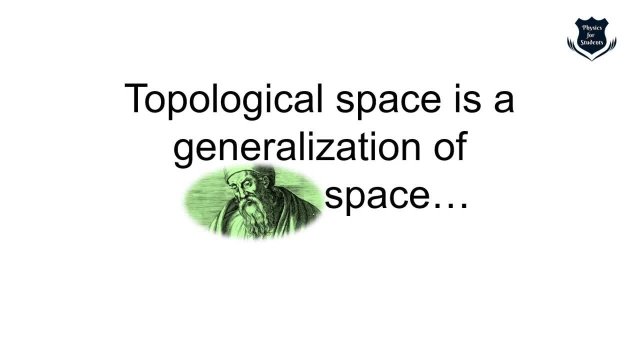 space is a generalization of Euclidean space right Now. once we say that topological space is a generalization of Euclidean space, we mean that we are generalizing the Euclidean space into better forms. Now, if you see that topological space are far-reaching generalization. 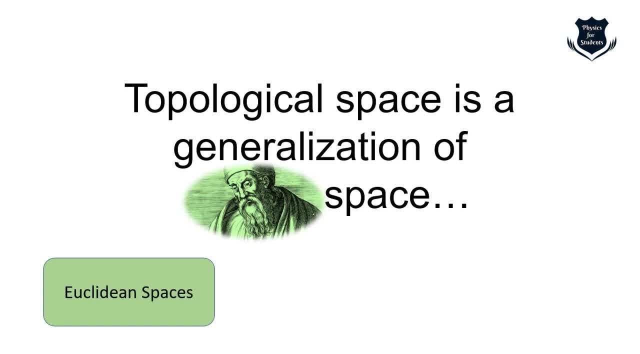 of metric presses, which in fact is a generalization of Euclidean space. then you can see that in turn is a generalization of Euclidean spaces, which is this: So Euclidean spaces gets more into metric spaces and metric spaces gets more generalized into topological spaces. 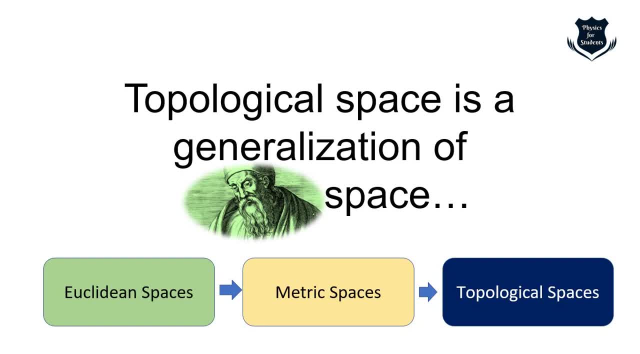 At this point of time. you might question that: what is the use? What do we do? The answer is simple: Simplicity. We want to define everything in a very simple way so that all those axioms, et cetera, can be generalized. 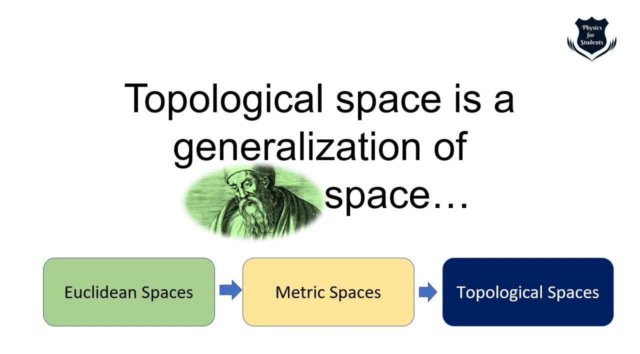 be understood in one particular theory and in one particular way. Now, when I talk of metric spaces, what I mean is by this: We have three points: x, y and z. The conventional way of measuring these points is by a non-negative function. We draw a line and we get this. 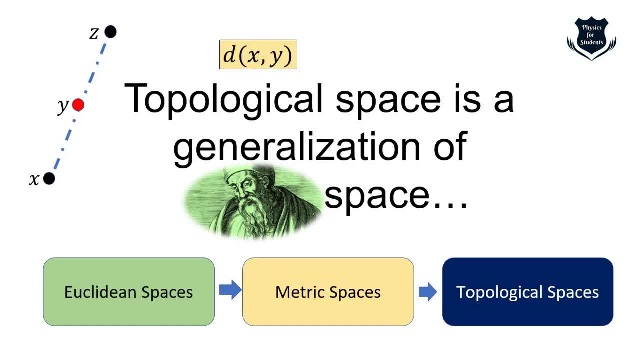 function d of x comma y, and we can further write as this: Here s is a set and d is a metric on s. So this function is no more and it is now being generalized The way we will look forward. So from Euclid we are moving to metric, metric we are moving to topology By metric, I mean to say. 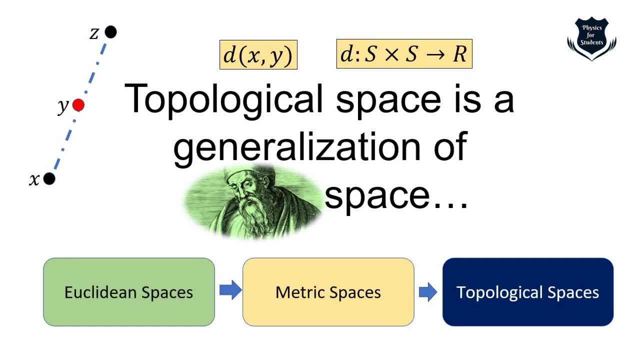 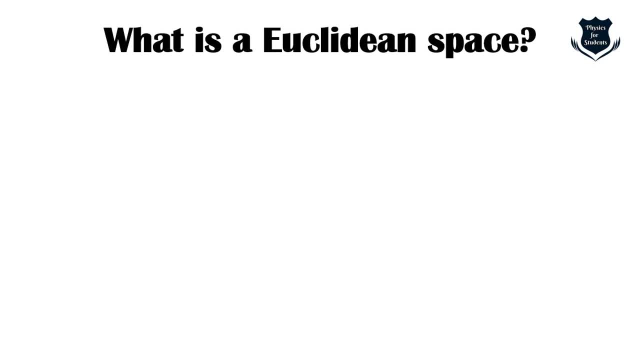 the typical conventional way of measuring points. Now, what is an Euclidean space? First of all, in order to move from Euclid to topology, or Euclidean space to topological space, we need to understand what is a Euclidean space. In order to explain the Euclidean space, first we need to understand that what is called a tuple 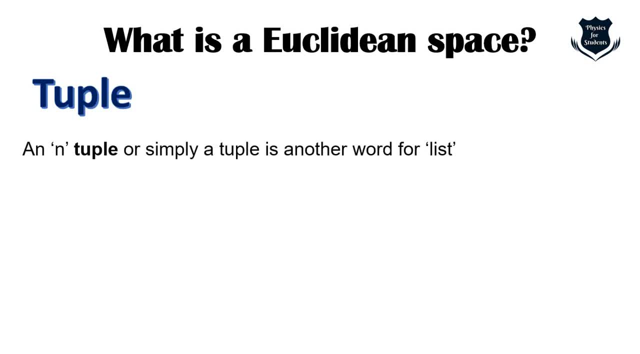 Okay. so here is the definition. An n-tuple, okay, or simply a tuple, is another word of list, or you can say it is an ordered set of n element. You can call it as a vector of n or of or n vector, whatever. So say, for example, these: we call these n-tuples, which are called points. This is a very 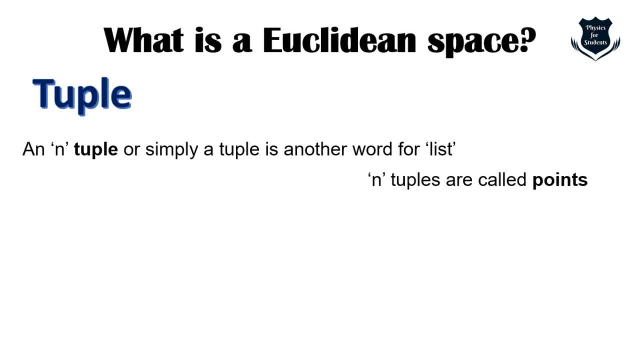 basic definition of Euclidean space. So these monad piers, triples, quadruple and quintuple, these are some of the examples of Euclidean space, examples of tuples, I'm sorry. And now see, in Euclidean n-space, also called Cartesian space, is the space of all n-tuples of real numbers, say x1. 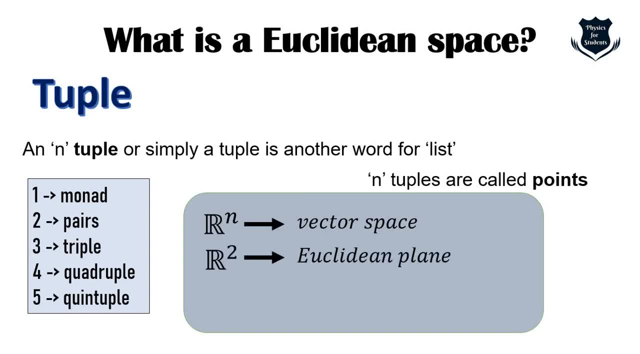 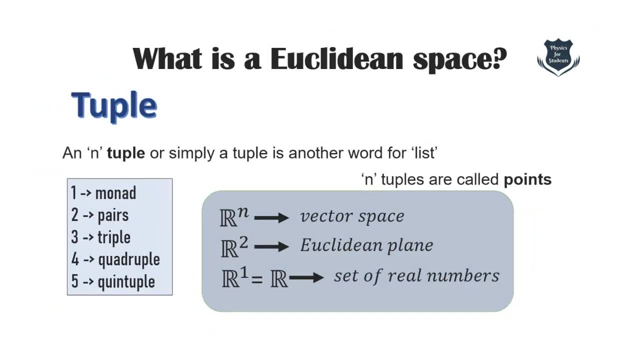 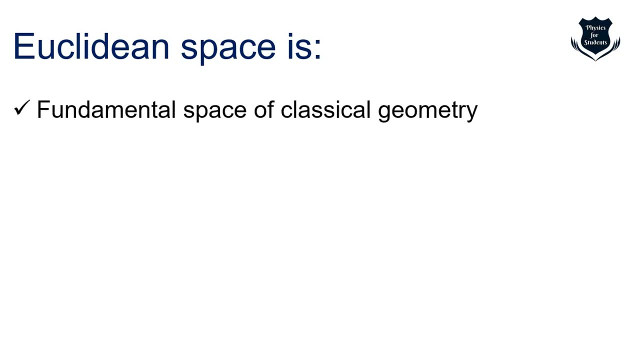 to x2, which leads to this R2, which can be called as Euclidean plane, and this can be called as a set of real numbers. So Euclidean space is 1. It is a fundamental space of classical geometry. We all know that It is a finite dimensional inner product space of over real number. We know that Now, line 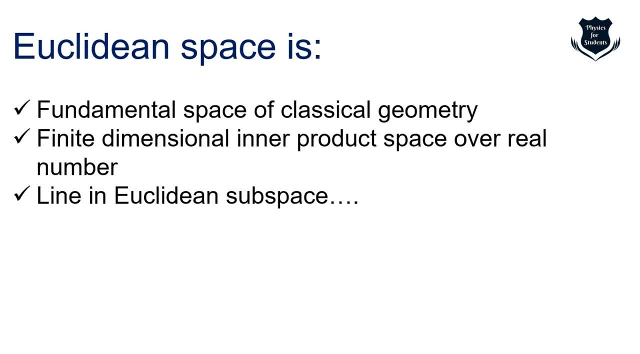 in a Euclidean subspace is of dimension 1.. Two subspaces, s and t, in a Euclidean space are parallel. they have the same direction. This is another point. The distance between two points in Euclidean space is given by this: Two non-zero vectors, v and u of e, which is a vector space, are perpendicular. 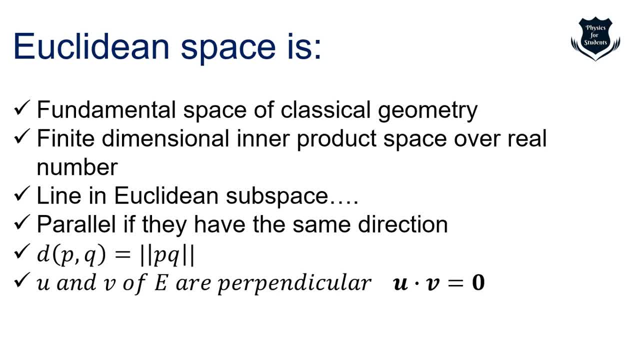 Yeah, so if the inner product is 0.. So this is just a kind of a very quick recap on the important points of what is in Euclidean space. Now there are other properties like angles, isometries, Euclidean group. Well, it would be too lengthy in this particular video. Now the 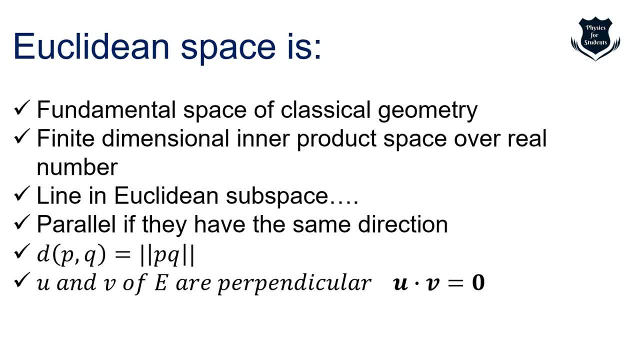 Euclidean space makes, sorry, the Euclidean distance makes a Euclidean space, and thus it is called a topological space. So you see that this topology is called this, Euclidean geometry. So you see that in Euclidean geometry we also have a topology. So this, this point should be quite clear. So 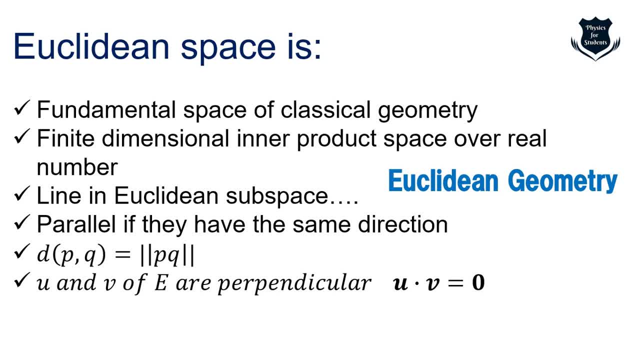 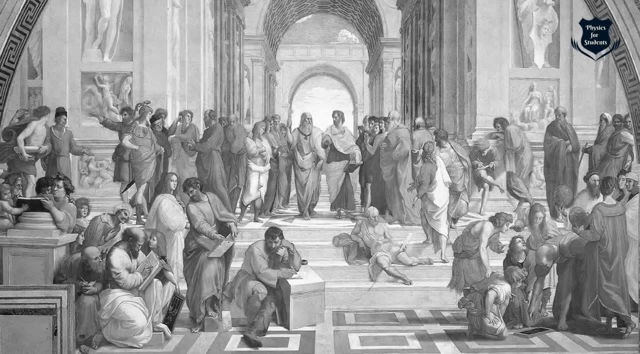 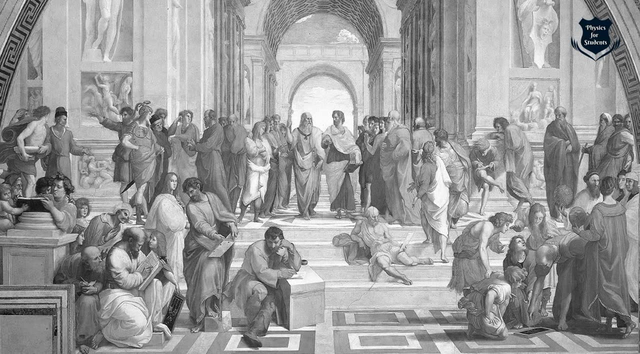 the Euclidean, make distance, make a Euclidean space and thus a topological space. So we have topology, which is a generic term in Euclidean geometry also. Well, those who are painting on connoisseur of art might have recognized by this time that what it is. Yes, you are absolutely right. This is the. 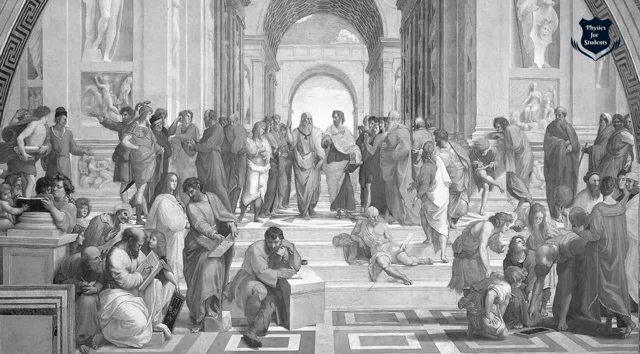 school of Athens painted by the famous Euclidean painter. This is the school of Athens painted by the famous Euclidean painter. This is the school of Athens painted by the famous Euclidean painter, Italian painter Raphael, around 1509 to 1511.. Now you might be wondering why I have taken this one. 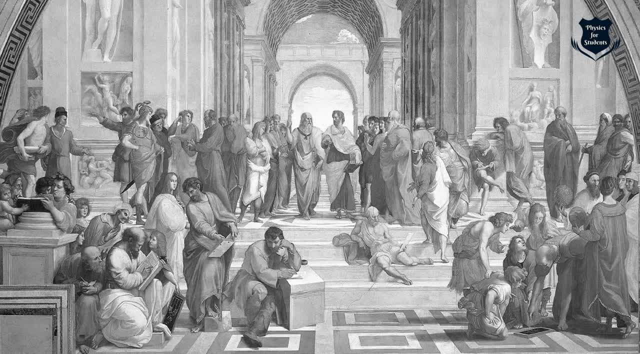 because here you will see everyone, right Aristotle, you can find, I think, the right in the middle with long beard, You can see Pythagoras, You can see Archimedes, You can see Plato, everything. Now, the basic idea of showing the school of Athens is that they developed axioms, and now we are going to 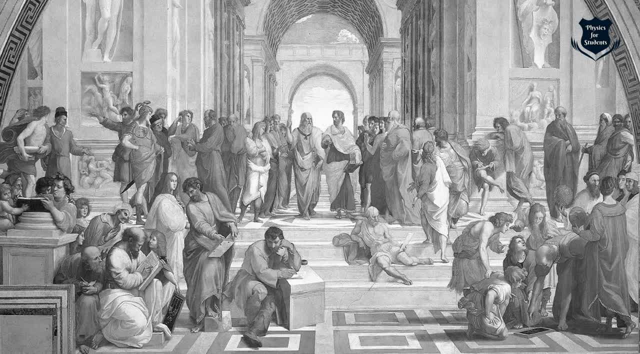 concentrate on Euclidean axioms. So we are going to concentrate on Euclidean axioms. So we are going to concentrate on Euclidean axioms. So we are going to concentrate on Euclidean axioms And how we can take it forward in order to understand what is called the topological axiom. This is a classical painting. I 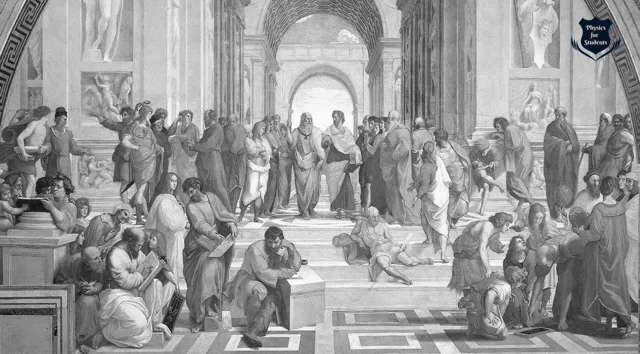 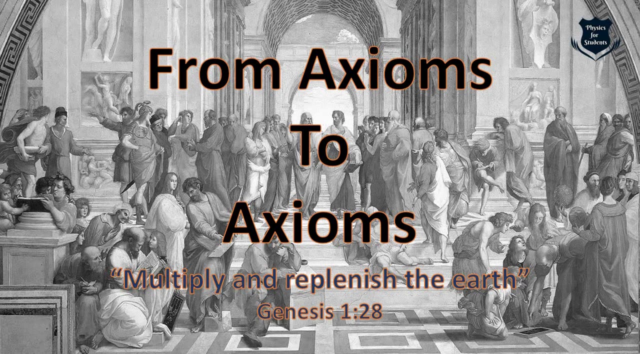 really liked it. But the simple reason is that all these people- if you can go into details, you will see they really develop certain axioms. So we can say that the Euclidean axioms really developed certain axioms. What we can say is that: 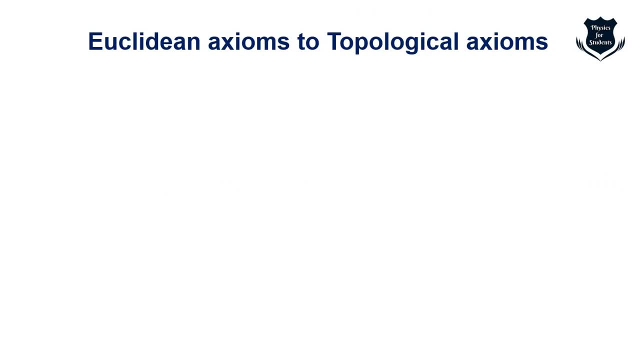 they really developed certain axioms. So we can say that they really developed certain axioms. So we are moving from Euclidean axioms to topological axioms. It would be easier for us to understand Now. see, topology is the abstract version of geometry. 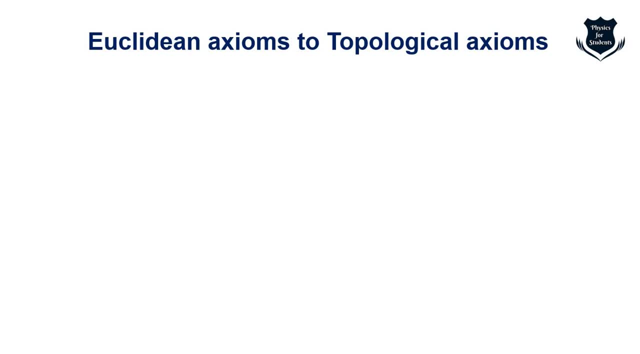 All geometrical shapes are topological spaces. We take some basic features of the geometrical spaces and try to figure out what will be the consequences of these features And what are the consequences Axioms. Then only we can get a very clear picture of geometrical results and their dependence on axioms. 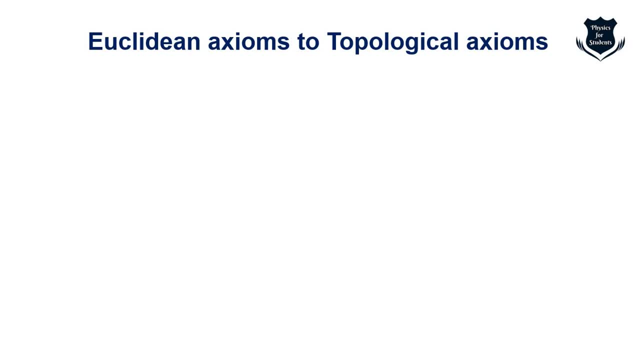 Now, mathematical proof, as you understand, is a very watertight argument which begins with information, proceeds by logical argument and ends with a proof. So to define topological space we need axioms, Otherwise how can we prove that? Say, for example, we start with axioms in Euclidean geometry? 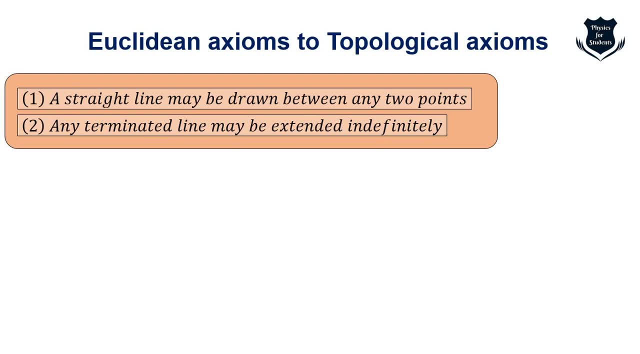 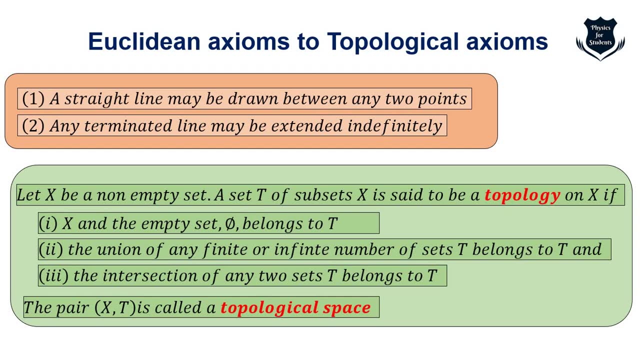 We have learnt it in our school days And then we move into what is called this. So on the top, which is in orange, is Euclidean geometry And this is the topological axiom. So you can read the bottom part. I think it is quite self-explanatory, but we need to go all through that. 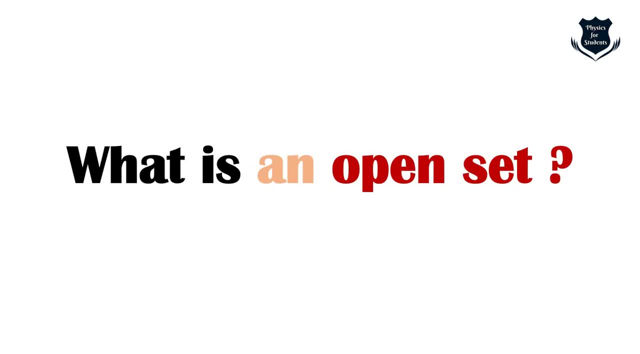 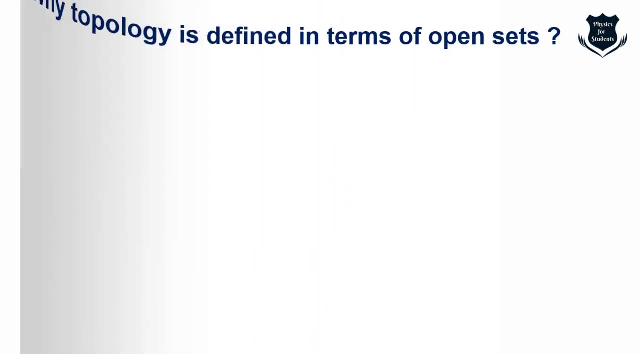 So now the thing is that we have all been doing this, but there is something important. That is why topology is called an openset. Now, in order to do this, we also need to understand that, why topology is being defined in terms of openset. 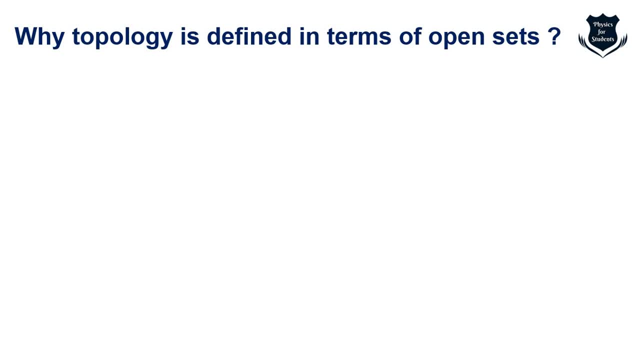 Yes, this is the pertinent question: Why topology is defined in terms of opensets. Now, one thing is that, obviously, as I told you that we are moving towards generalization, We are generalizing every notion, from Euclid to topological species. 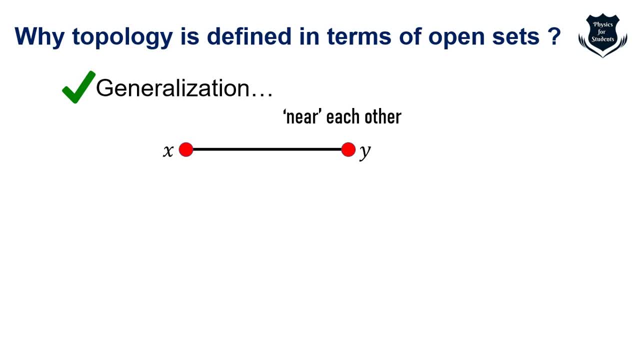 Yes, Yes, that this right. so these two points, x and y, which are quite near to each other, right, and we can define it by a function, DXY, which we are not doing. right, so we are. you see the purple arrow, this DXY, the function is being replaced by open sets. so why topology is defined in terms of open sets? answer. 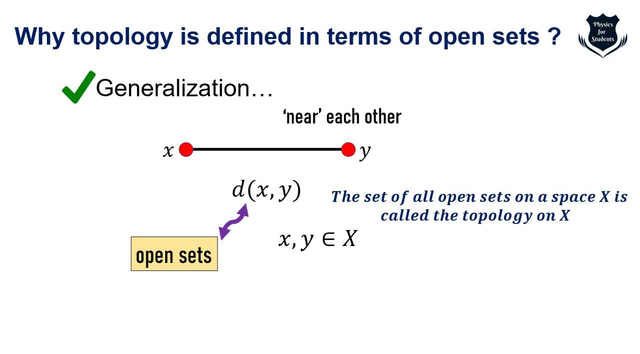 is simple. the concept of the function is now being replaced by open sets. the set of all open sets on a space, X, is called the topology on X. so this is the reason that topology is defined in terms of open sets. so matrix distance equation we are not using, and this is what we call is a more. 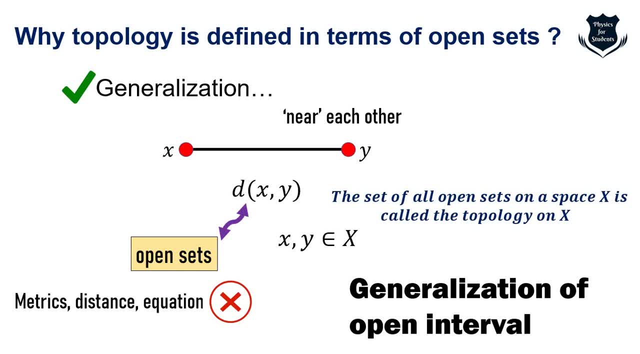 generalized form of those you have read. you must know what is an open interval. so this is the definition, or I would say the right definition, of the function DXY, which is defined in terms of topology, which is defined as using matrix and sectionation, square and speaking ofivanpa. 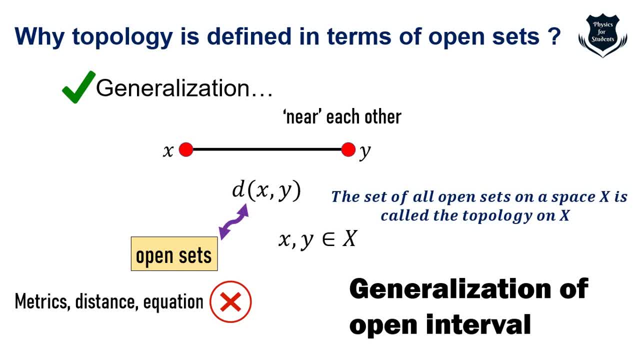 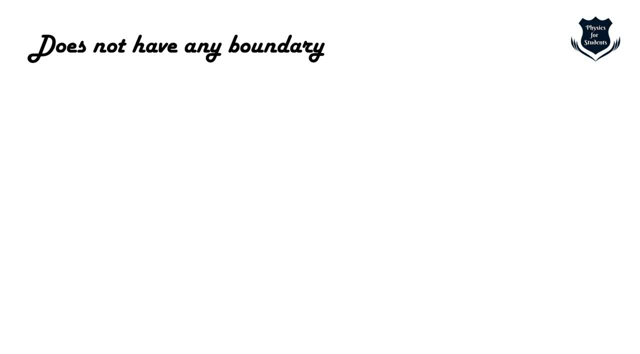 formulae. we do know that why 하게 are steht in the agenda is defined in terms of the open set ropology we are seeing many rage is at its worst, but rather the crux of the topology, that why it is different in terms of open said because we are not using matrix distance in equation. we are generalizing it in open set, which can be taught of a generalization of an open interval. so will come to this part. once we understood the blocks of building, blocks of the topology, you go back to the axiom. we look into this. so we have to look into the mathematical proof of the axiom once. 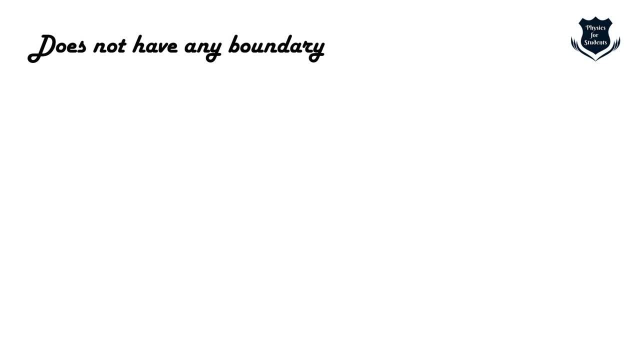 was the axiom. puisque lepsi history, they have a graph where the Goldenément, Charlotte found gross, are satisfied, we get the proof. now the basic thing that we need to also understand is this: so, as you see, in topology, the entire generalization, which is an open interval for real number, is an 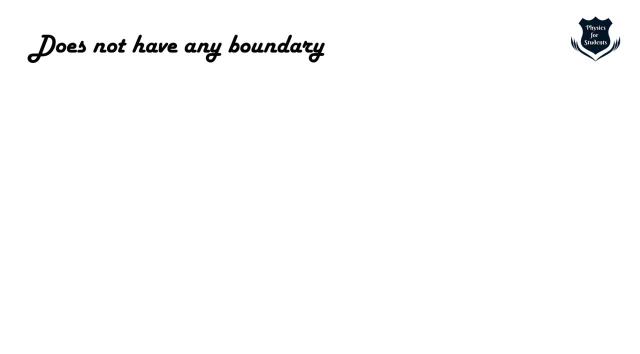 open set. so in most of the text that you go through you will see the topology is defined in terms of open set. you can think of an open set as a set that does not have a boundary right. so here is a circle right, and we get two points: x and y. we know the and now we know that an open. 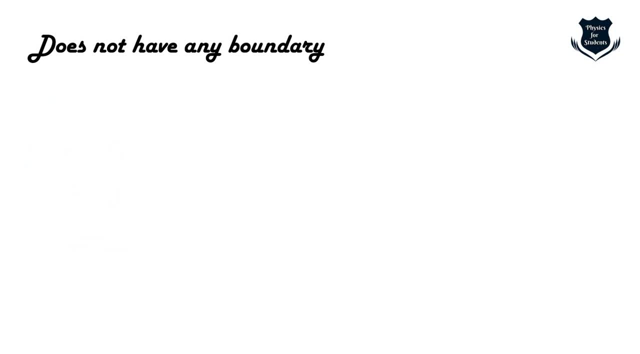 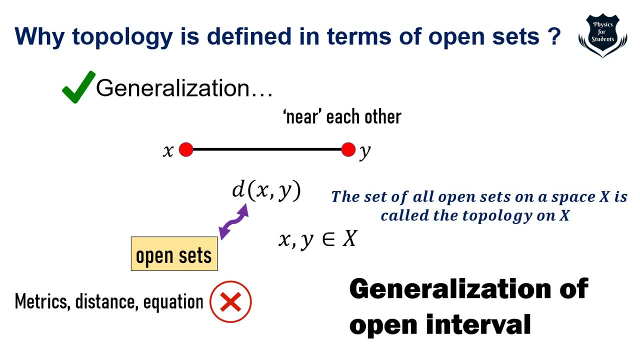 set is one which does not have any boundary. i thing if we can go back to this part, you see that this is basically the definition of open set. I would like to tell you that we can think of near each other if there are a lot of open points that contain both points the other way. 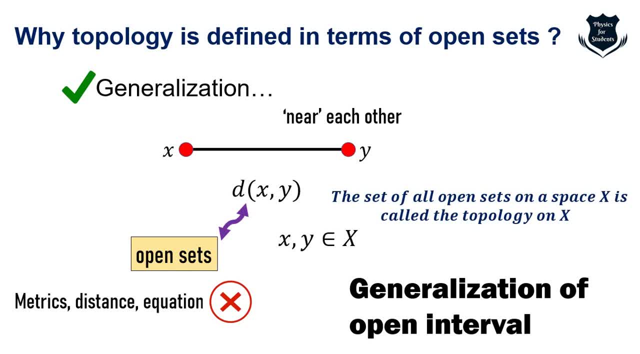 is also a cue to the entire total set. so the hypothesis of the set of close setora over powders are basically two points behind one another, while we we have a loop and for each of the two points. So true that if there are two points that are never contained in the same open set then obviously they are very far apart. 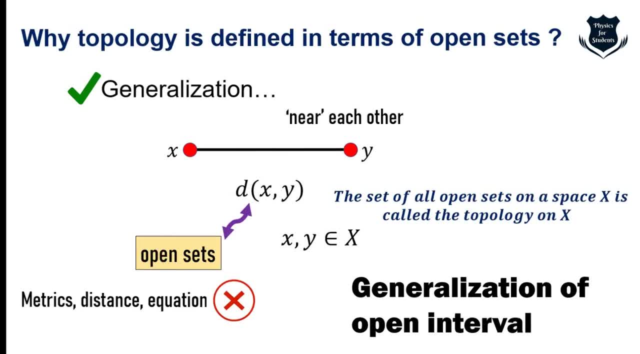 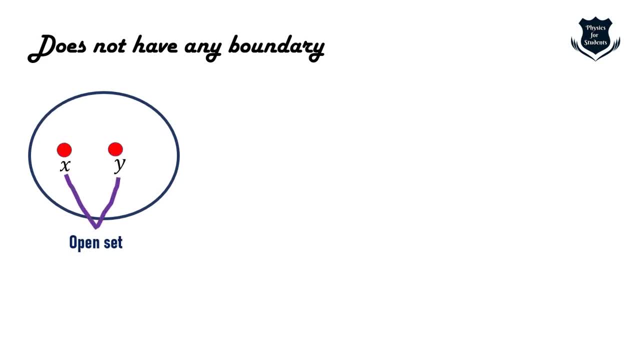 So in topology we do not use matrix, distance, etc. Now, if I take this particular figure, which is a circle, we know that there are no open sets, So we get this X and Y. So here is something which have two points. 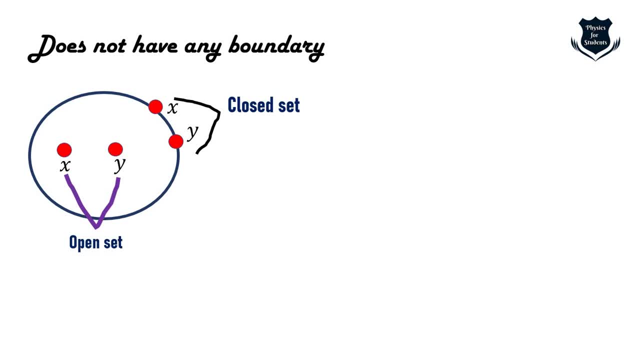 And now you see this. OK, so X and Y, that lies within the disk but not outside. Where is the open set, The red dots, X and Y, which is within the circle, and various. This one is outside, which is within the boundary, is called called a closed set. 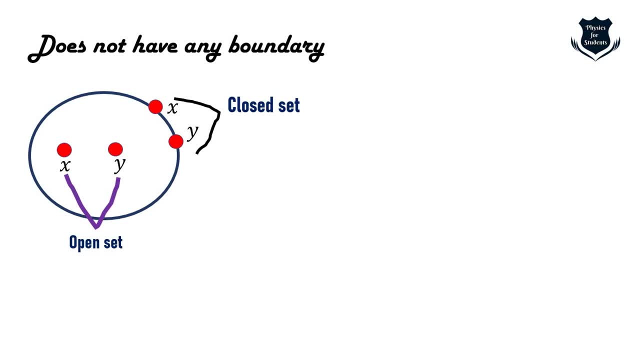 We are not concerned about closed closed set, We are more concerned about open sets. So we have a circle and we have two points, X and Y, that lies within the disk but not outside, is an open set and forms an open set. But this one which lies on the boundary, 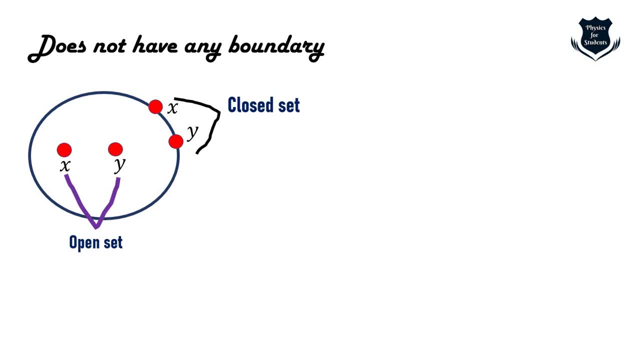 So we have a circle and we have two points, X and Y, that are not open sets, and it is called a closed set. In order to explain things further, you can think of this: So the green area around the red circle is an open set which has satisfies this equation. 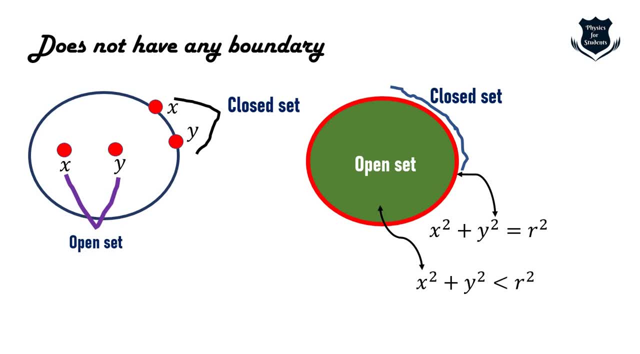 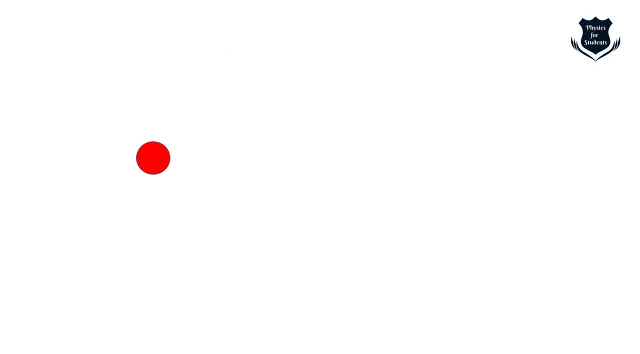 And this part is the closed set Right. So this is the open and the closed set concept, which has got no boundary. in one way, We can think of it as an open set. Now, here is a small example: A small perturbation or movement, but it should lie within the set. 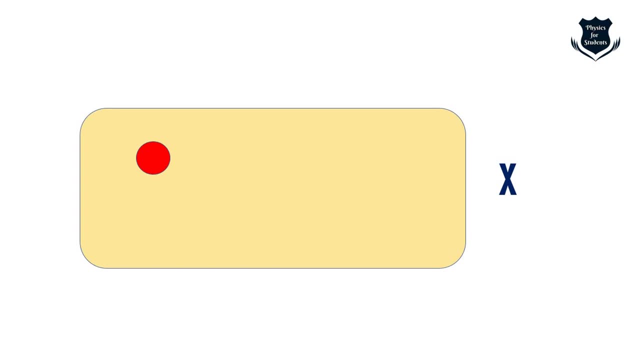 So here is something which I have magnified it. And then here you cause a little bit of perturbation of the red ball. It goes here, here, here, here and here, But you see everywhere, wherever it is going, it is not leaving the set X. 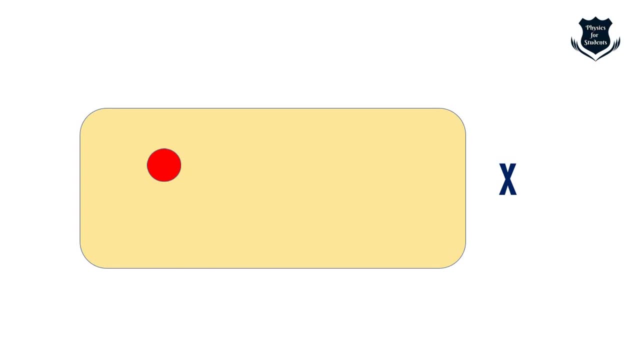 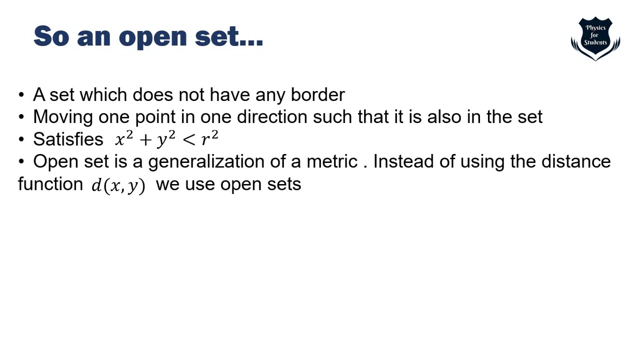 Right. So this is also something which is concerned and you can think of it, something that it will be easy for you to visualize. So what is an open set? more precisely, a set which does not have any boundary, which we have seen moving one point in another such that it is also included in the set which I've just shown in the animation satisfy. this open set is a generalization, obviously, of a matrix. 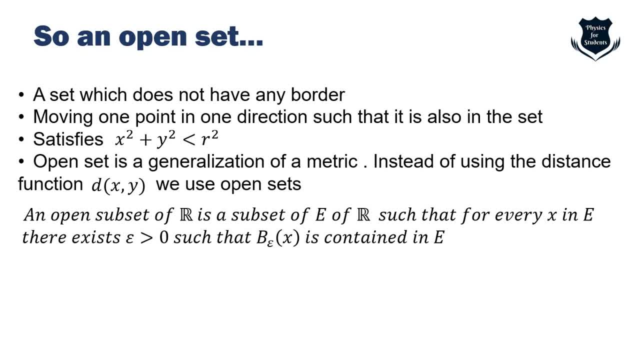 And instead of using this function, we use open sets. and open set of R is a subset of E of R, such that you can read this forward. And yet this epsilon is a number that contain an E And, for example, the open interval two comma five is an open set. 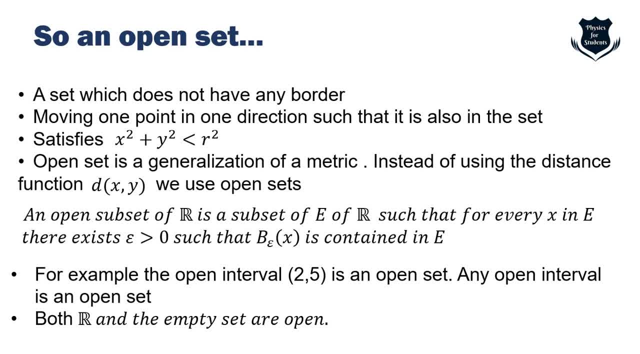 Any open interval is an open set. So both R and the empty sets- that is a real number- are open. We can expand on that but this is not the right time. So just it is a few important points of defining what is an open set. 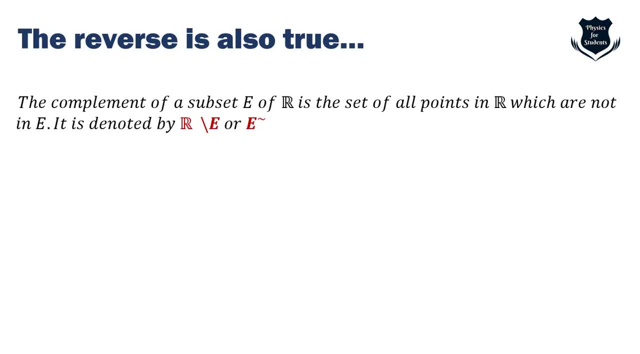 Now also the reverse should be true. That is the complement of the opposite of subset of E of R. It is a set of all points which is written either by R, black slash E, or you can write it as E tilde. 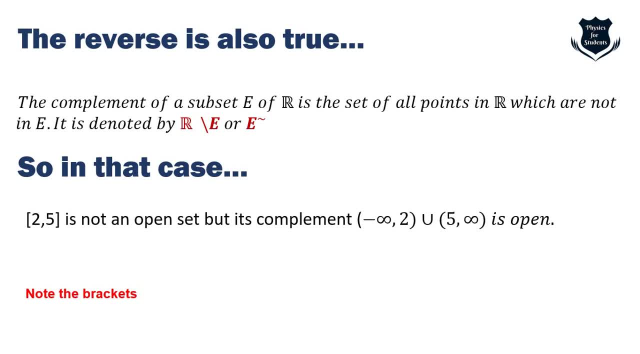 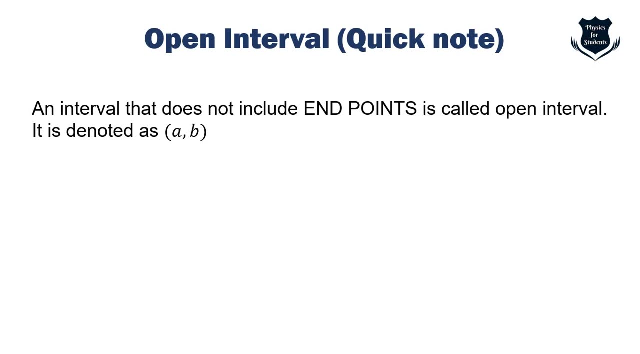 And in that case two five is not an open set, but it complements minus infinity two and it is a union of five to infinity is open. So this is a quick note on what is an open interval. I won't spend much time. 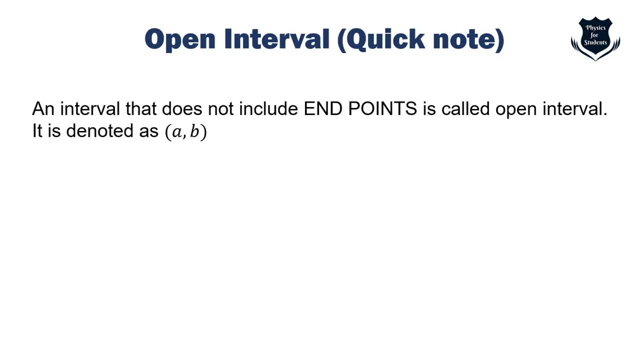 It doesn't include endpoints, right, It is denoted as E comma B. So you just see that we all know that. you know this. braces zero comma two. this brackets are called intervals, open intervals and square brackets are called close intervals. 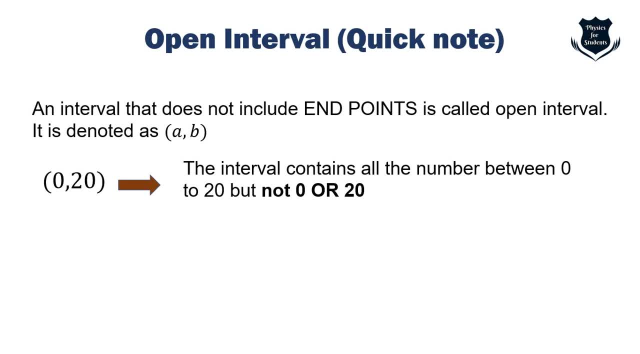 So the intervals containing all the numbers between zero to two, but not zero or 20.. So it can be written as this or it can be assigned also as this: So a circle includes the end values and a circle which is filled up does not include the end values. 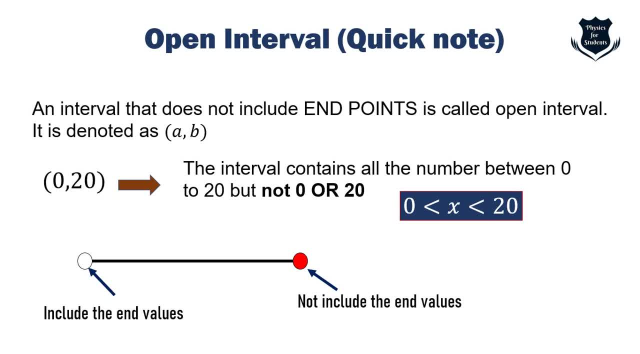 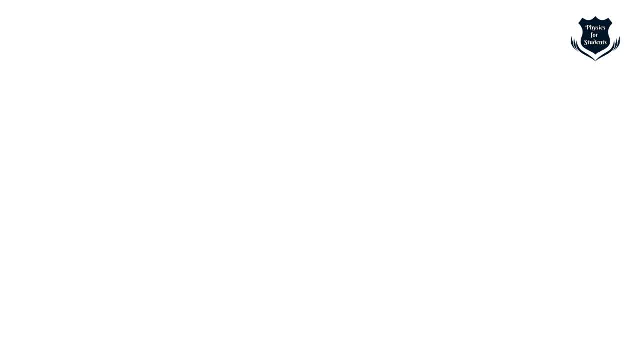 This is very preliminary. I just thought to give you a Quick idea of what is an open interval, Right? So, as you might have noticed, that in topology we are talking all about has a point in intersection. So topology in which the intersection of any family of open set is open is called an Alexandrov topology. 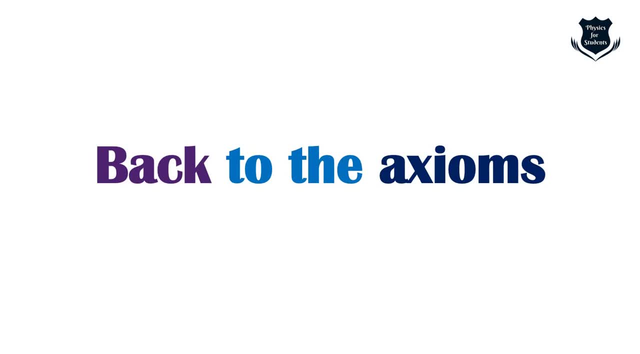 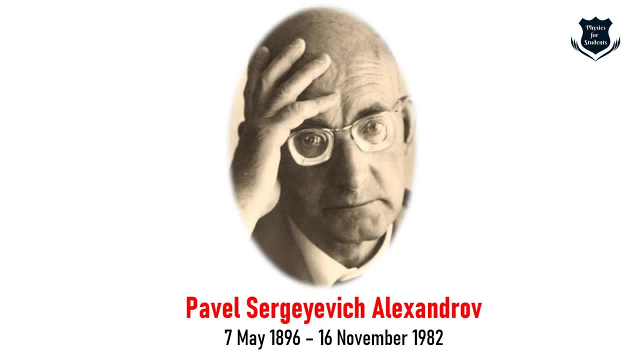 Well, we will just look into it. What are you trying to mean Now, this Soviet mathematician, Pavel Sergeyev Sergeyevich Alexandrov. he contributed immensely on the topics that we are reading Right, And we call them as Alexandrov topology. 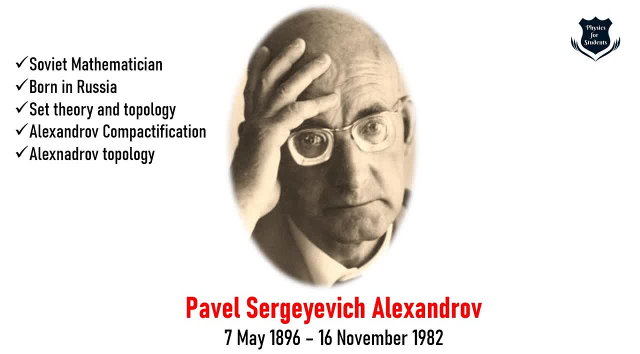 So you can just have a quick look on his contributions. He was a Soviet mathematician born in Russia, Set theory and topology. He made quite a big contribution and is known for Alexandrov compactification and Alexandrov topology. Now Alexandrov actually made his first major mathematical success in 1915. 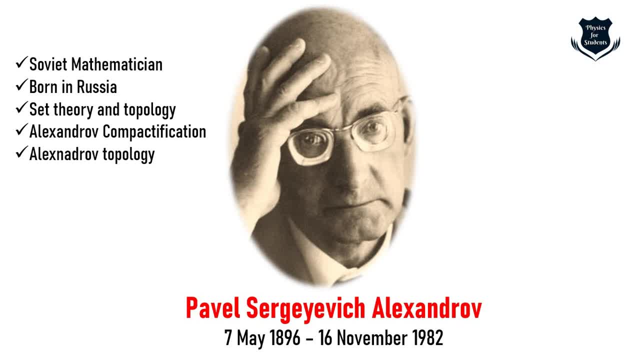 In set theory. he worked with Felix Hasdorff and developed what we called today is a point set topology or a general topology. So in 1920, he developed combinatorial topology. He was the president of the Moscow Mathematical Society. 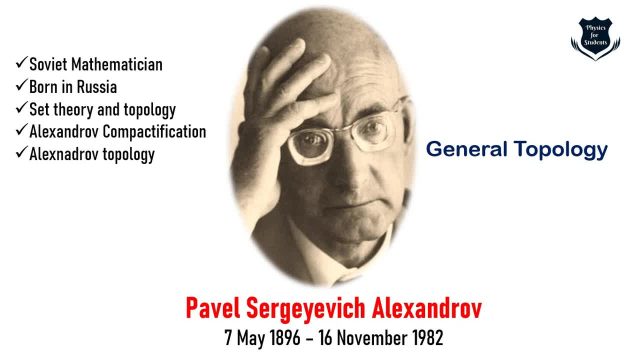 Vice president of the International Congress of Mathematicians and full member of Soviet Academy of Sciences from 1953.. The basic understanding of this gentleman is that whatever we are learning, the general topology or the Alexandrov topology, is because of this. So I just thought to give you a very quick idea of who this person and what is his contribution in terms of topology is. 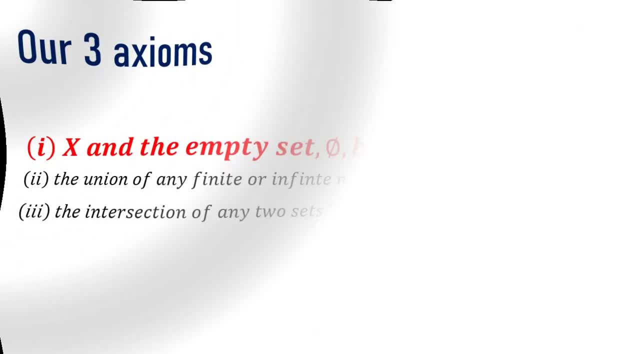 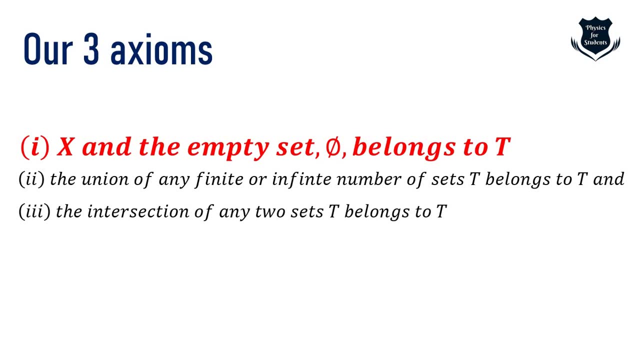 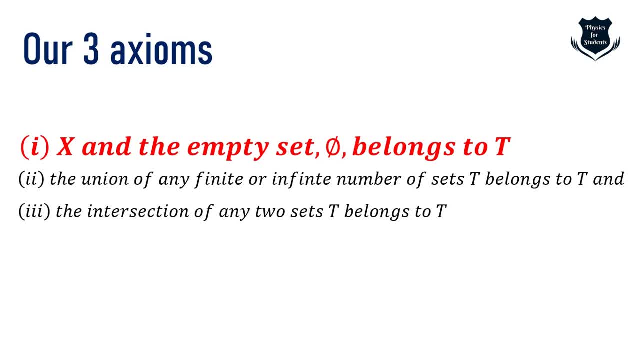 And you can comment on this. So what do we get? So, we get the three axioms right. So now, what we are going to do right now is that we are going to take two approaches Right. One is a very intuitive approach which might not sound very correct mathematically to you. 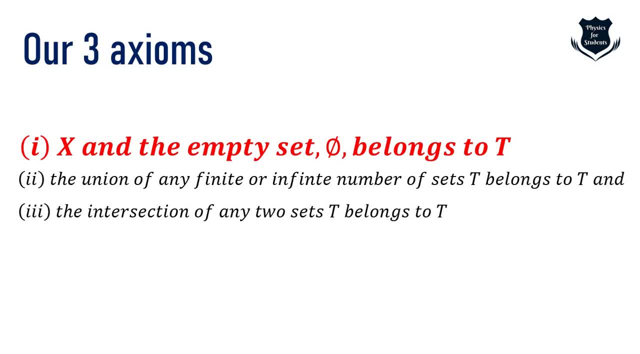 I will again repeat these words. It might not sound mathematically correct to you, but it is important to have a visualization of how we're going to prove these three axioms. So first we are going to take this x And said phi belongs to t, and then we will go for the second and third. so the first approach would be a. 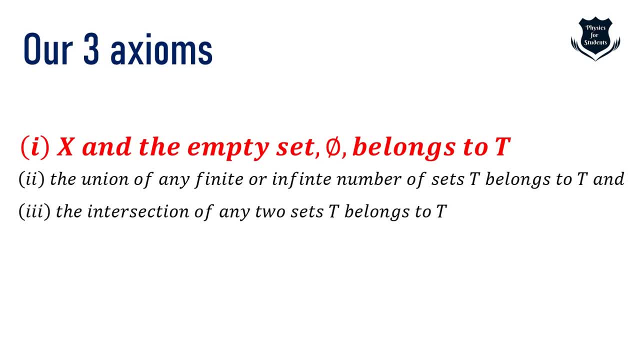 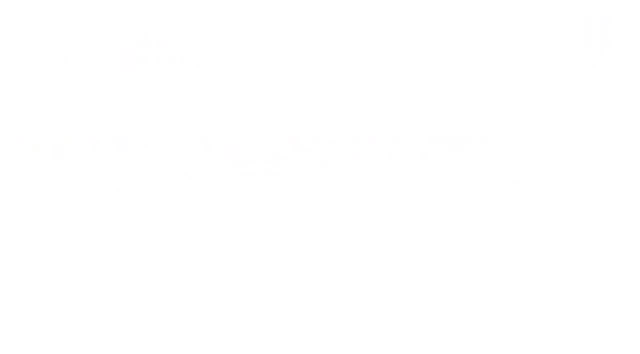 intuitive and a non-mathematical approach, and then we will look into what we call is a more of a mathematical and we'll give examples on that. so here is a figure, right? so this diagram shows set with l x. sorry, it shows set x with elements a, b, c. topological space is a set example. 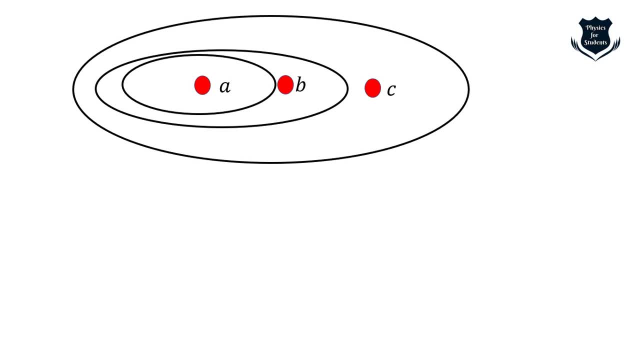 x plus a collection of subset x that satisfies three axioms which we have seen earlier. this of subsets is: this collection of subsets is called a set x. so here is a diagram and i can say that the oval- you can see these oval shapes. they represents open sets. so i can call this: 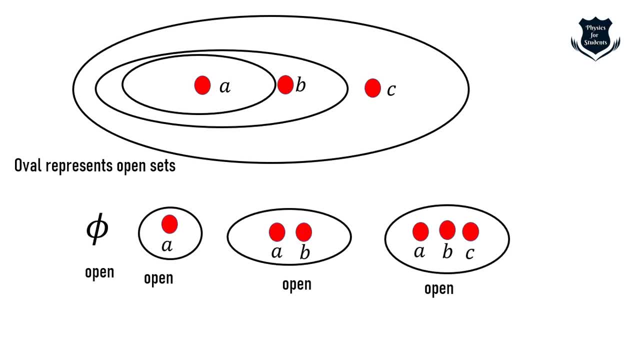 phi, this one, this and this as open, and, if i uh, now the set on the extreme right hand side which we will see, is actually the set x itself, because it contains the elements a, b and c. now, if we write typically in our conventional curly bracket, then we can get this right. so you see that, uh, you can. 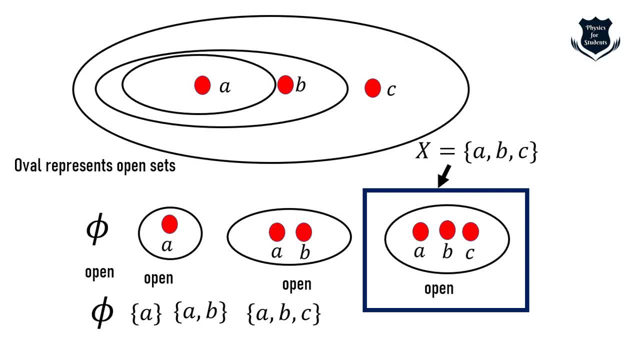 check it out. going back, that axiom one is satisfied as x equals to within curly bracket x, a, b and c and t is in the list, so x and the empty set phi belongs to two is satisfied right. so again, as i told you, it's a very intuitive approach coming to the. so what we got? we got the first one, green ticked. 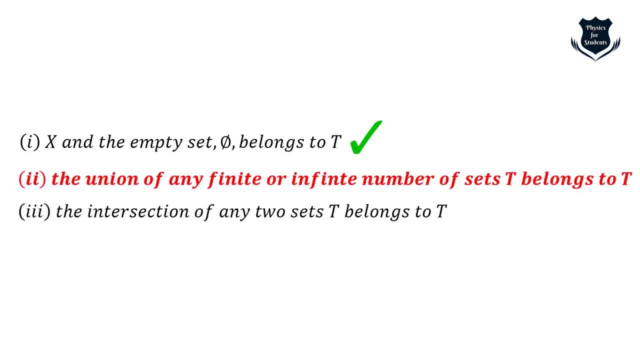 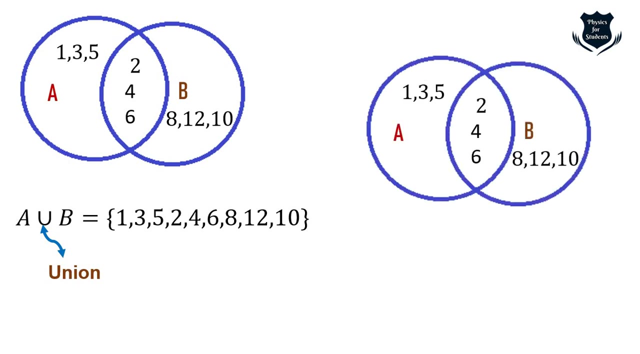 that means we are done with the first. we are going to find out the union of any finite or infinite number of sets. t belongs to t. now what we are going to do is that we are just going to take a quick, brief look on those who really know they can ignore this part. what is in union and what is a intersection? i think things. 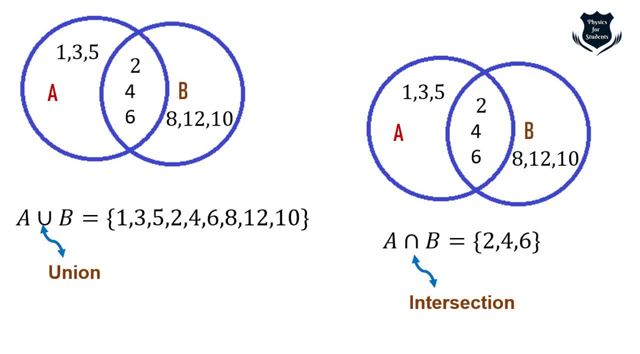 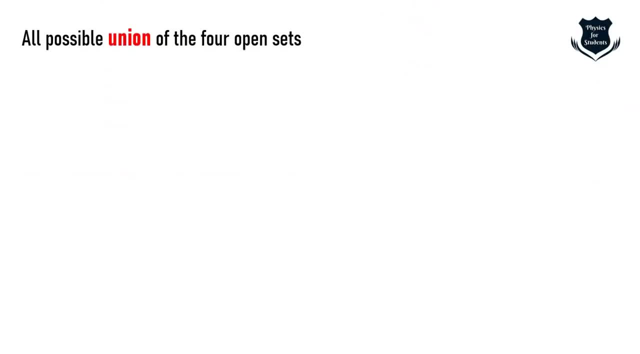 are quite clear so we don't need to waste. uh, i would say we need to take more time on understanding union intersection. now in the first, axiom is done. so what is the second? it is all possible. union of the four open sets. so if i take the list phi, a, b and c, so i can just take an example, a is an union. 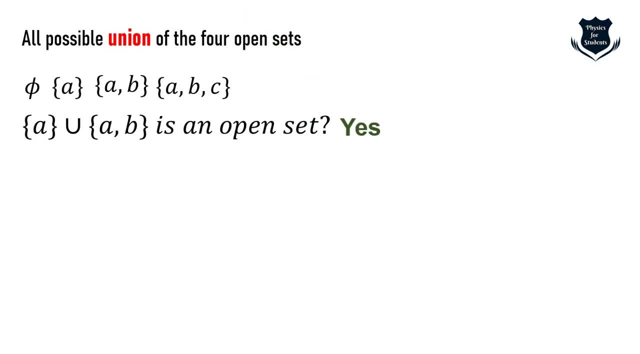 of a- b. is it an open set? definitely it is an open set. right, we can further take x as a union of a set which is equal to x is already open. for example: x union a, b equals to x. we can further take another example: phi is the. 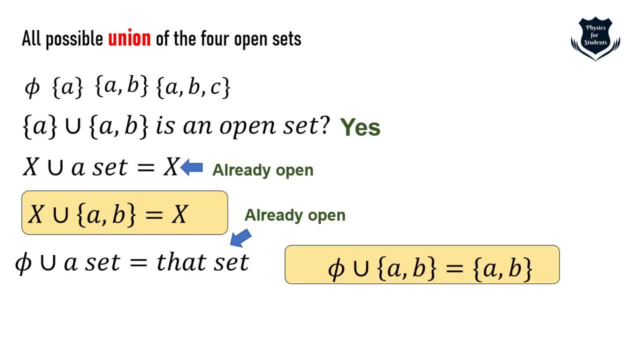 union of a set which equals to that set, for example this one. so from this what we get is that the union of any finite we have taken for these, these numbers actually, just as an example is- belongs to t and which belongs to t, the sets t belongs to t. 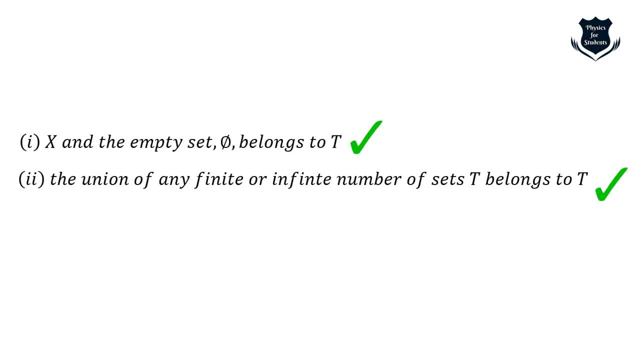 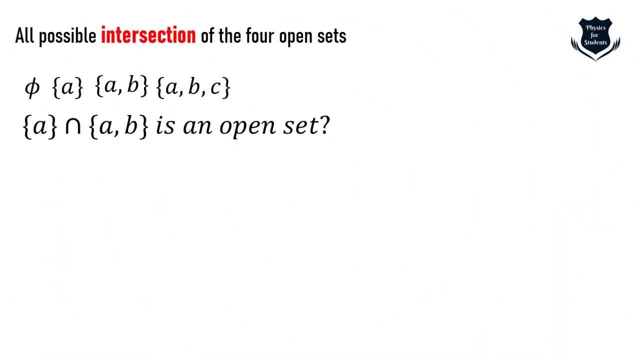 so finally, we have done with the first two. and then we are left with this: the intersection of any two sets t belongs to t. so we will go with the same approach: all possible intersections. we take the list and then we say whether it is an intersection. yes, it is an intersection. 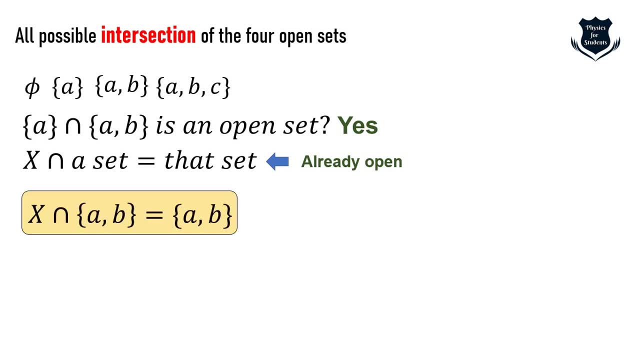 we take, for example, x intersection: a set equals to that set is already open. for example, this and phi is a intersection of a set equals to phi which is already open. so this equals to phi. that means we have also proved the intersection of any set, two sets. t belongs to t. so what we have really done. 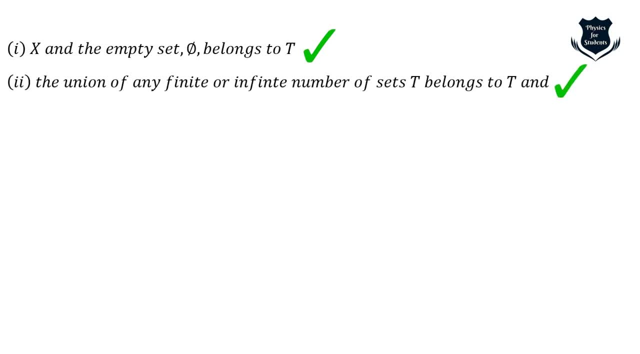 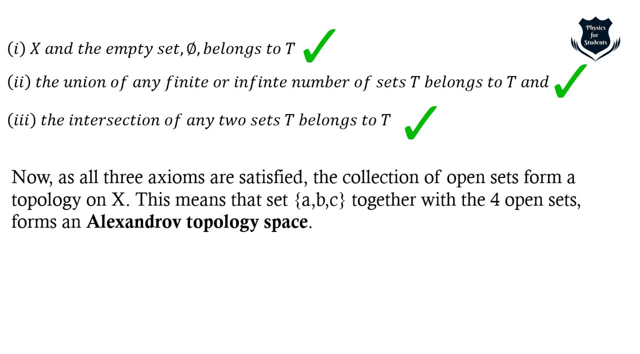 is that we have proved the first, the second and the third part, so now we can tell that all three axioms are satisfied. the collection of open sets form a topology on x. so you see, we are defining precisely what is a topology. this means that sets a, b and c, together with four open set. 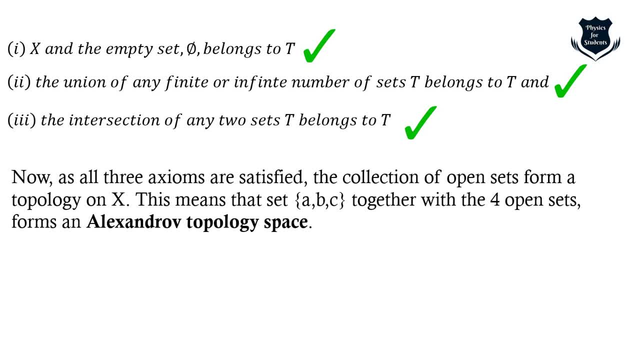 forms an alexandrov topology space. i am i i try to make things a little bit more specific- so i mentioned alexandrov's name, so you can call it as a topology space. so the pair x- t is called a topological space. so we will now take a few quick examples. 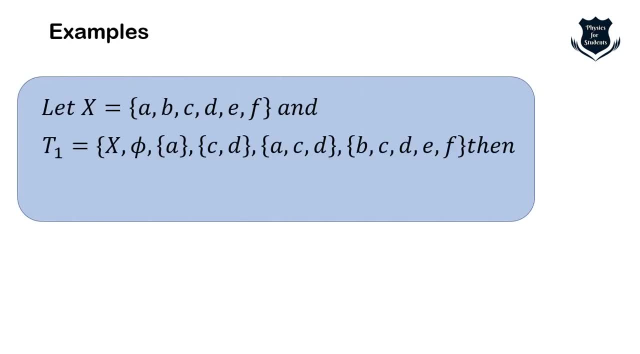 before we end this video. So we take something like this: x equals to a, b, c, d, e, f, these are the elements and t1 equals to this. Then t1 actually is a topology on x, y as it is satisfied. 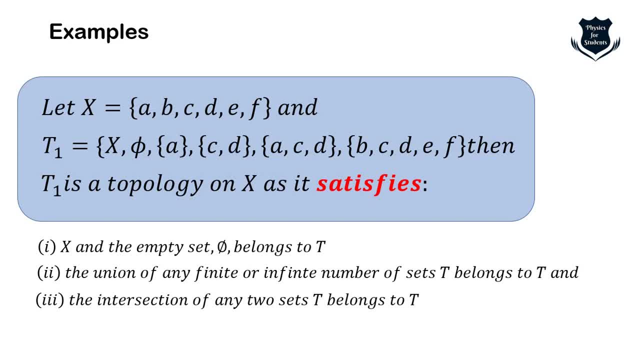 1,, 2 and 3.. So you can now understand why I was telling that we need to first understand intuitive understanding and then go for the exact numerical one. So this one is a topology, because it satisfies the bottom three points, or the axioms. The second example would be something: 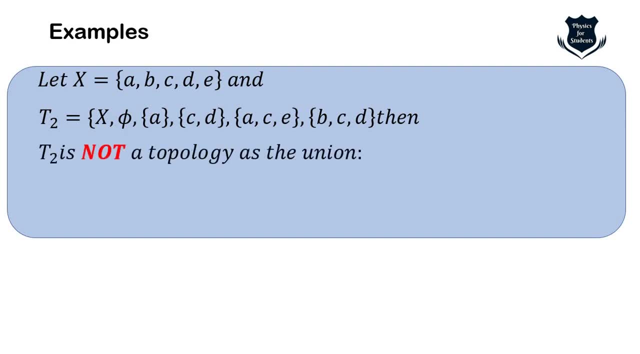 like this. and then it is not a topology. Why? Because the union of c, d, union of a, c, e, two members of t2 doesn't belong to t2 and hence it does not satisfy these three axioms. So 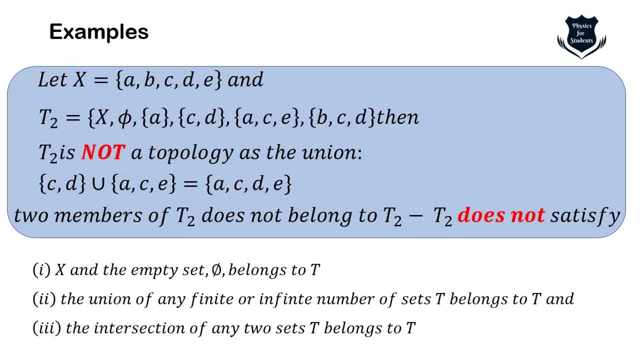 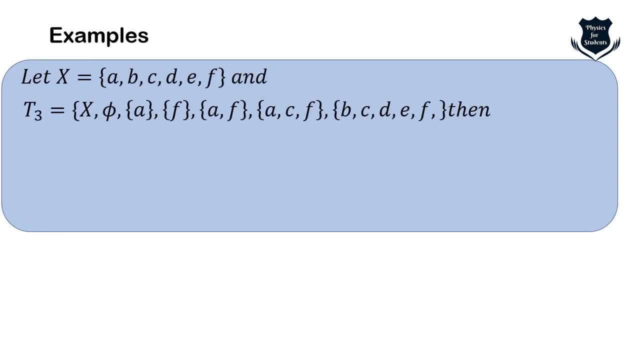 one of the axioms we have seen which is satisfying this union. this is not satisfying. We take another example, these elements, and we try to form a kind of an intersection. It is not Why? Because two members of t3 does not belong to t3. Obviously you can see the intersection c and f, So it doesn't. 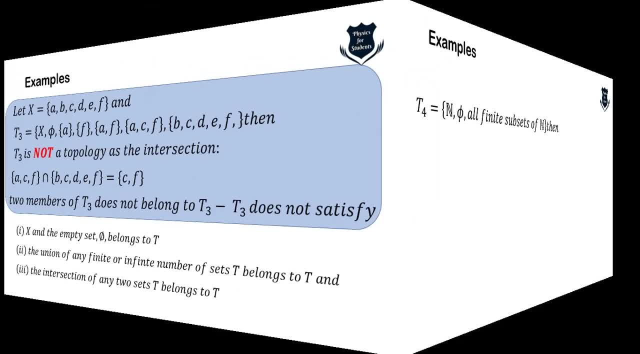 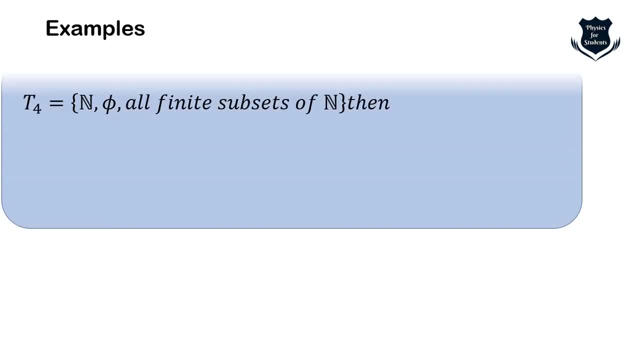 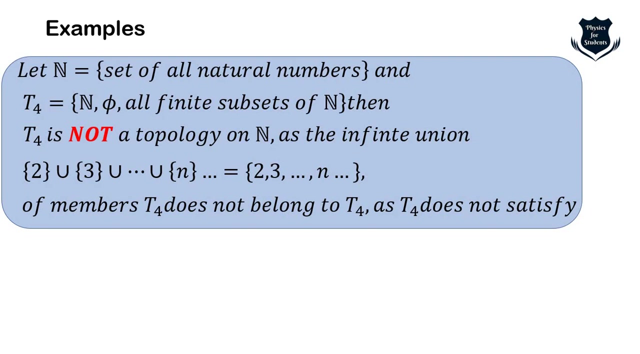 satisfy these three axioms. We take a further example, which is a more generic one. t4 actually equals to the numbers n and finite sets. Then n be a set of natural numbers, Then t4 again is not a topology, as the infinite union which goes dot, dot, dot, Members of t4 does not belong to t4 and 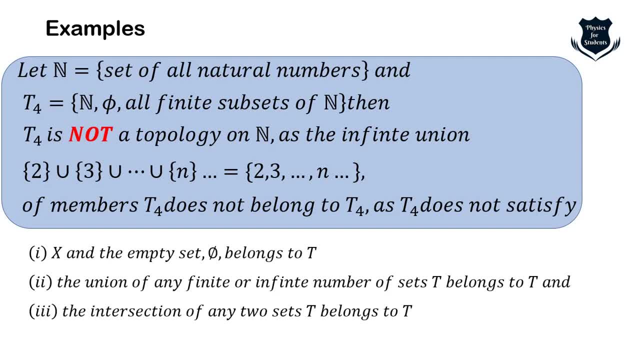 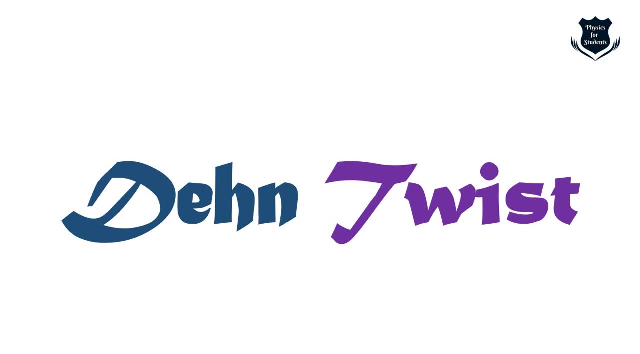 hence t4 does not satisfy these three axioms. So this is how you actually try to prove the axioms in order to define what is a topology, What is a topological space. We have come to the final part of the video, which is called a. 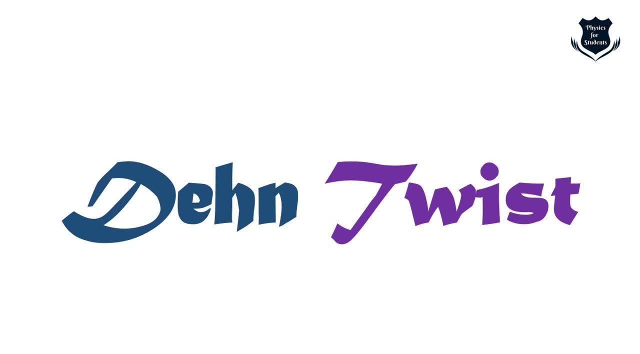 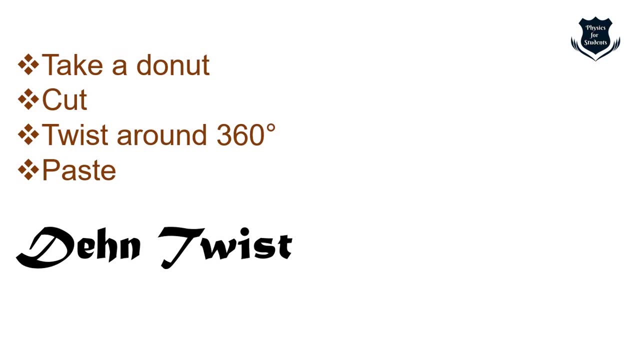 dent twist. As I told you, dent twist is a typical way in which you can take a kind of a donut and you can cut it, twist around 360 degrees, paste it, and this is called a dent twist, and the original form or the original points are never restored, So you can do a dent twist. I just wanted to. 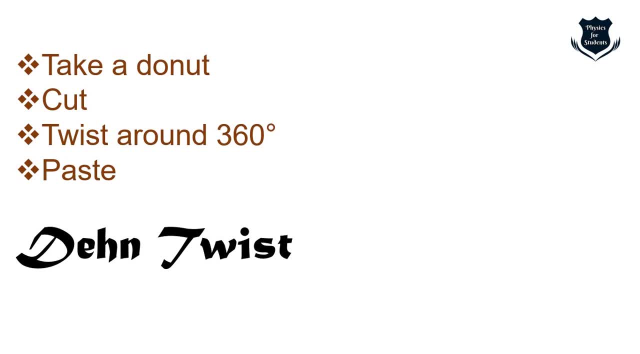 tell you that gluing and cutting are two different things. So you can do a dent twist and you can cut whatever you want. you can also do a dent twist. If you do dent twist by using a parent of your child, that is not allowed in topological space. 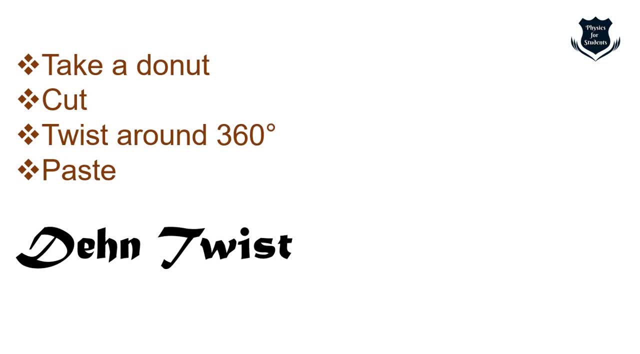 it is a wrong notion. It is very much allowed if you are using a dent twist. So it is a kind of a self-homeomorphism. and on homeomorphism, the last part, that this paragraph in blue is actually a technically definition of dent twist, I am not going too. 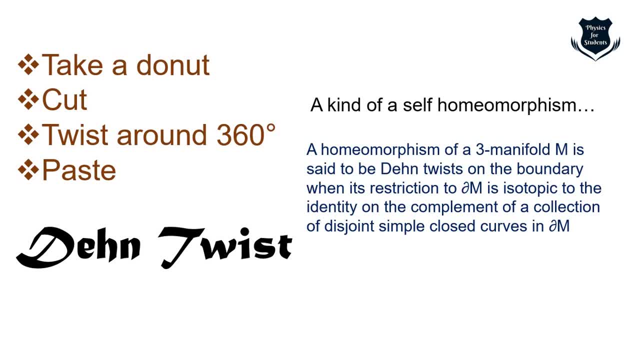 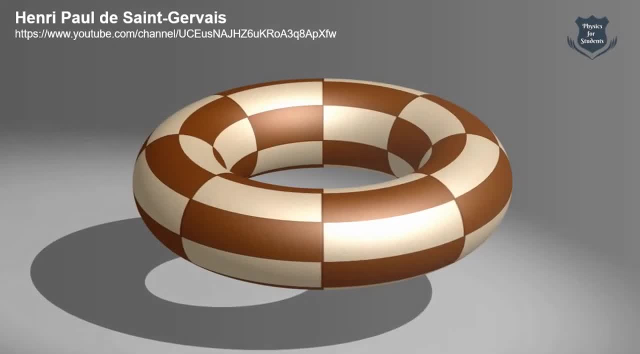 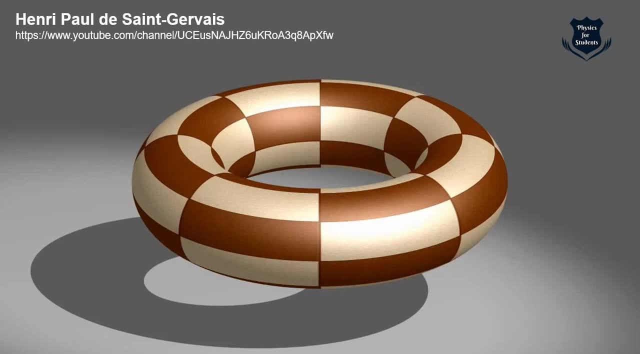 much into dent twist because it is a totally different kind of a subject. Now I would like to show what actually dent twist is through an animation. alegria-z is obviously not mine. I have taken this from a French first gentleman's channel and I have shown the courtesy. so here is a doughnut right and you get rotated. 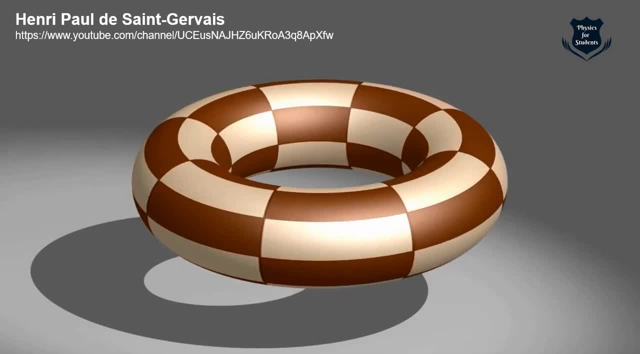 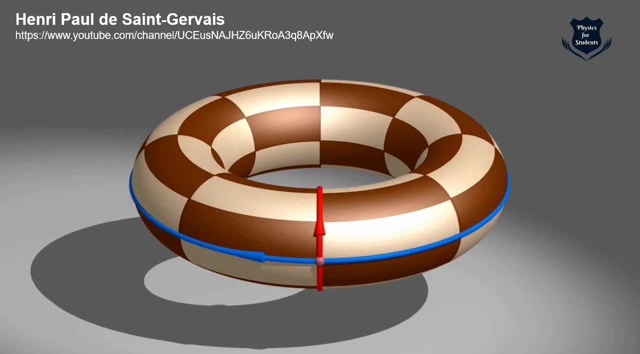 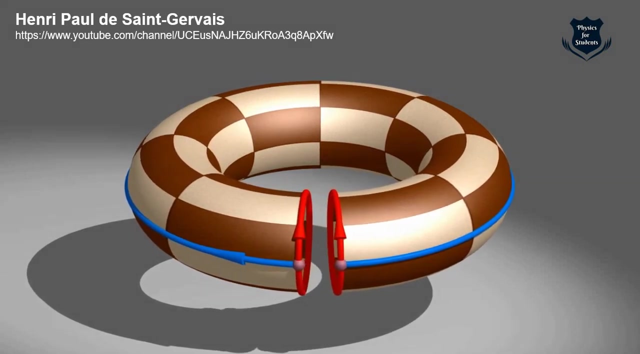 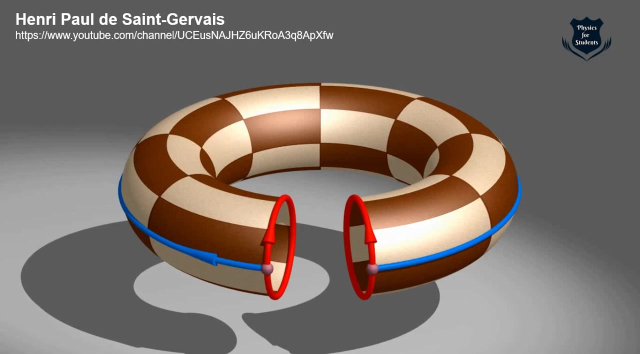 right now, you see the red lines which are coming. so what it is happening? it is splitting out or it is cutting out into two parts. here it goes. now we twist it and you see how the blue lines are changing, and after that, what we do is that. 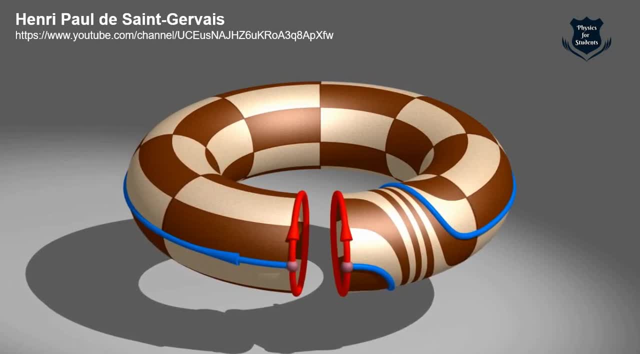 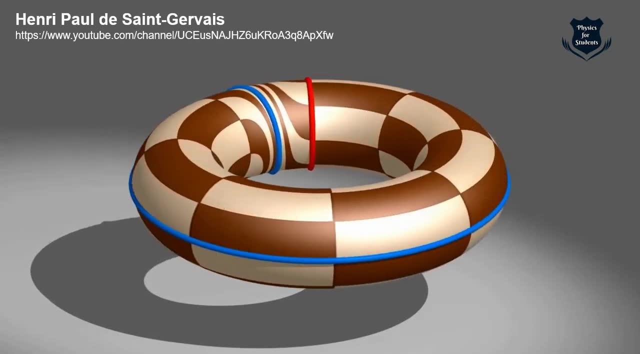 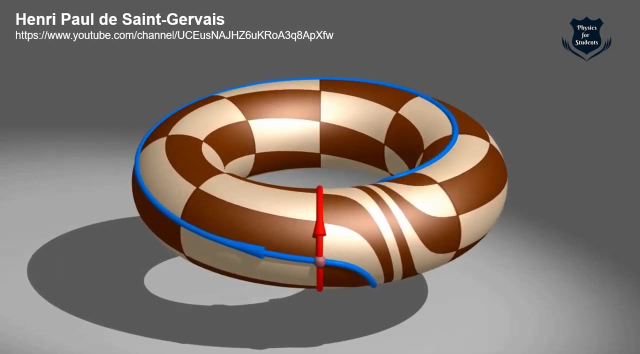 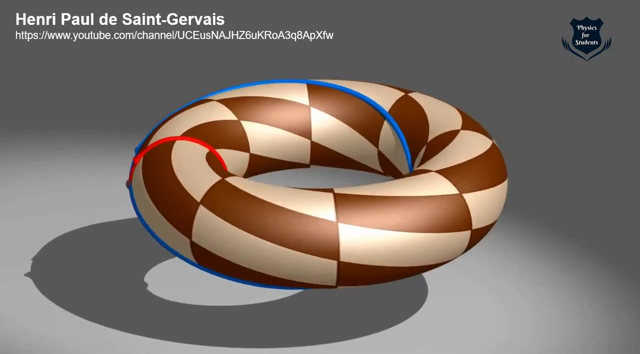 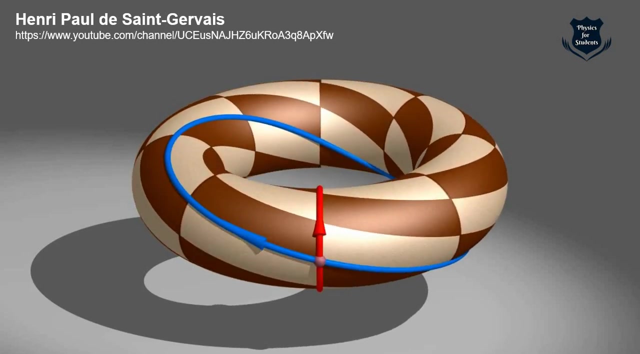 we do a rejoining of the points together and then we rotate it and then we twist it right. so this is a typical kind of an animation which I have taken from Henry Paul, and this actually shows what is the dent twist. so that is a typical kind of an animation which I have taken from Henry Paul, and this actually shows what is the dent twist, so that 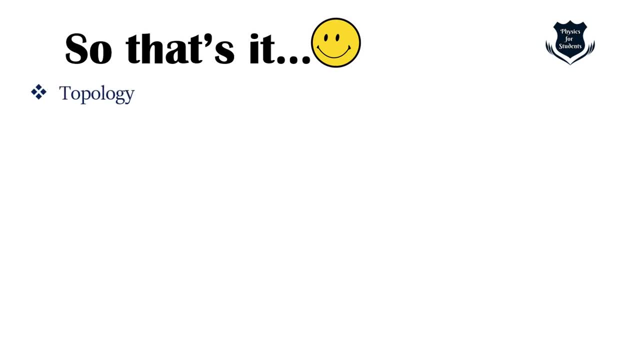 that's it, so the first part of the video. we have learned what is a topology, what is a topological invariance- that is, a property which doesn't change. what is homeomorphism? how, from Euclidean space we have moved into topological space, the water open sets, water open intervals, and a little bit about